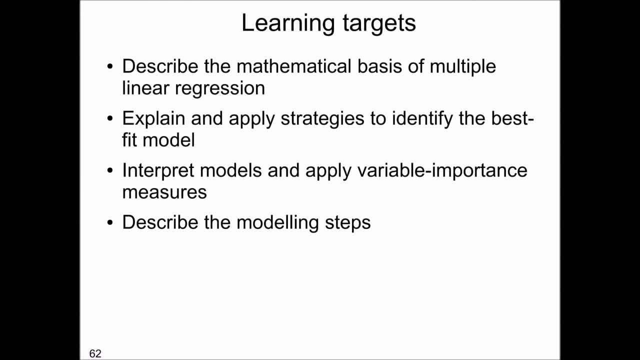 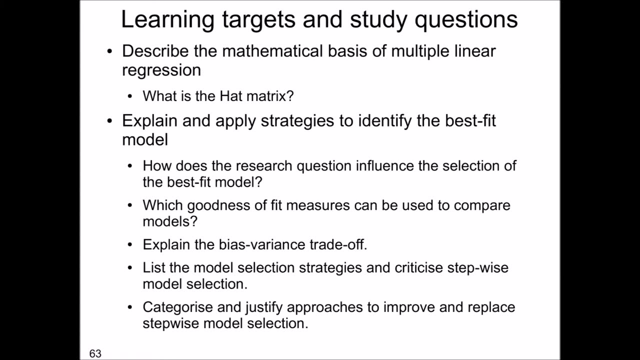 and apply variable importance measures. Finally, of course, the ability to describe the modeling steps needed in regression analysis. The learning targets are associated with study questions. these you see here and you can go through them and check, based on these study questions, whether you understood the material. 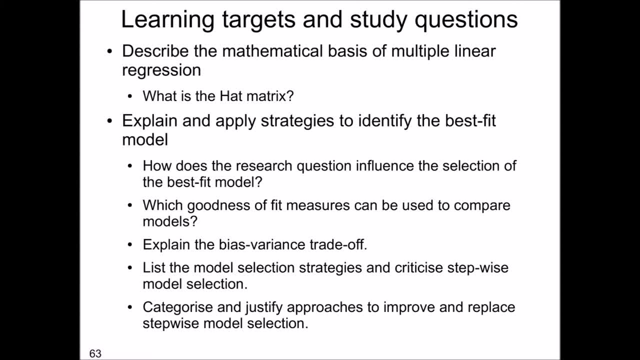 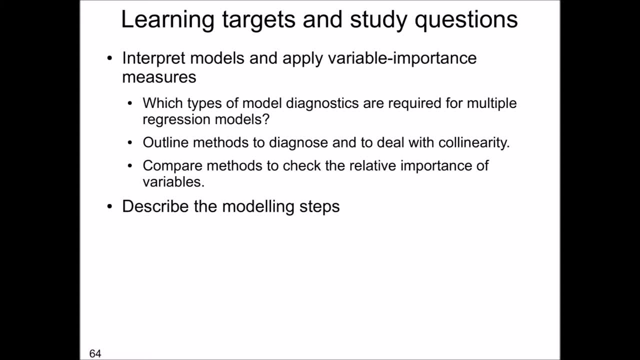 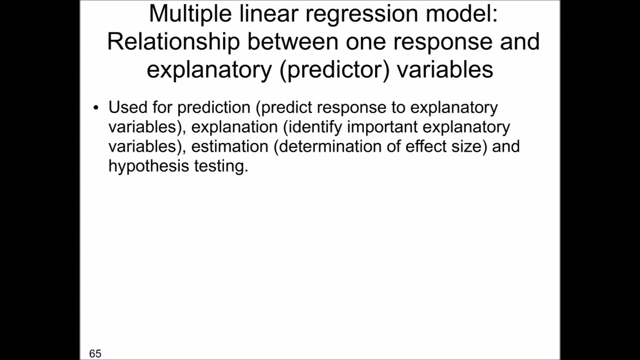 of this session. Same holds for this slide. Carefully read these questions and whether you can evaluate the modeling steps. So a linear regression model consists of one response variable and multiple response explanatory variables, also called predictor variables. These variables are used to predict this response. These models are used for different purposes and different aims. 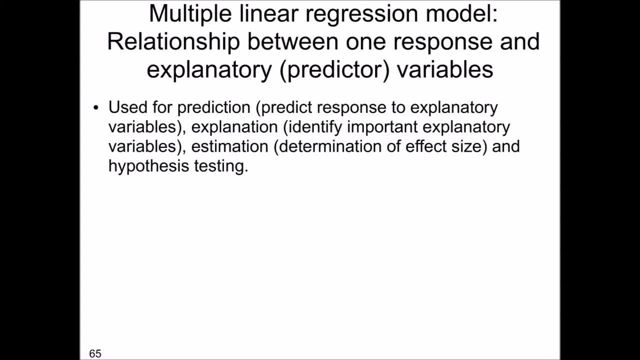 You may have, for example, the aim to predict something. You may want to predict the distribution of a species based on climatic or environmental variables. You might want to explain a phenomenon, so you will identify the most important variables that explain something. 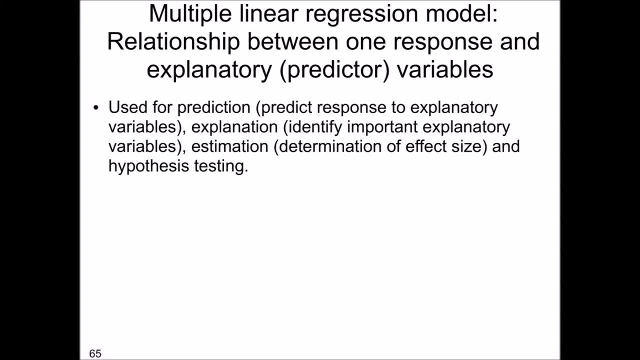 I will give you an example soon. You may want to estimate so to determine an effect size, For example the effect of fertilizer on freshwater species diversity or on the growth of plants. And finally, we might want to test a hypothesis, For example whether a relationship really follows an assumed. 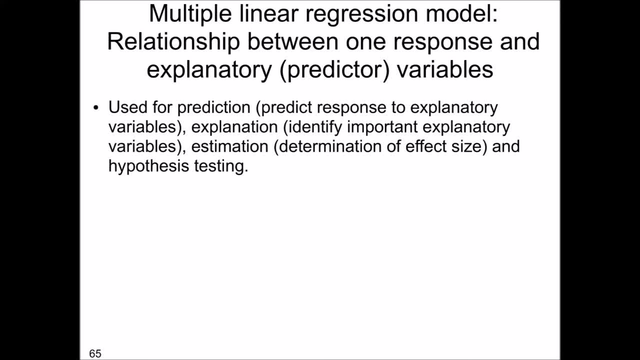 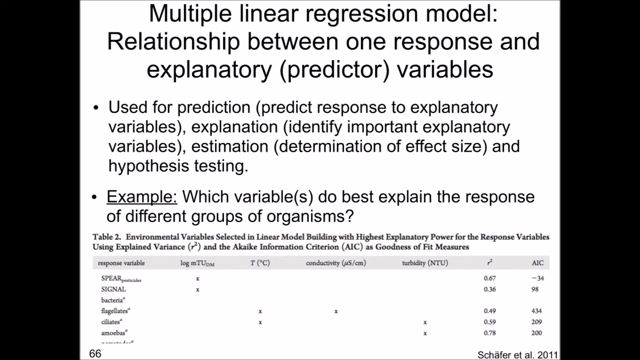 correlation coefficient, An example of the metabolic theory of ecology. There is a certain assumption of the size of the regression coefficient between the log-transform metabolic rate and temperature and other variables, But I won't go into details. So the example relates to a field study in Australia where we assessed different biological endpoints and looked at the effects of pesticides and other variables of invertebrates and microorganisms. 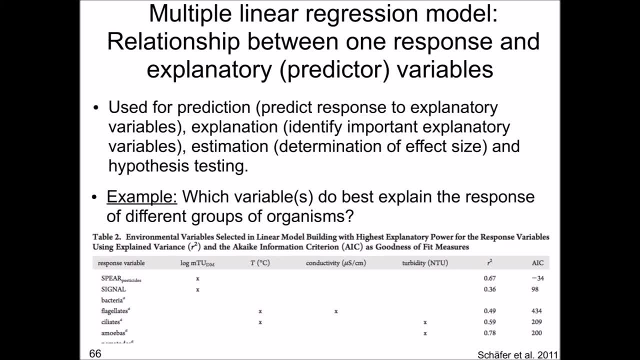 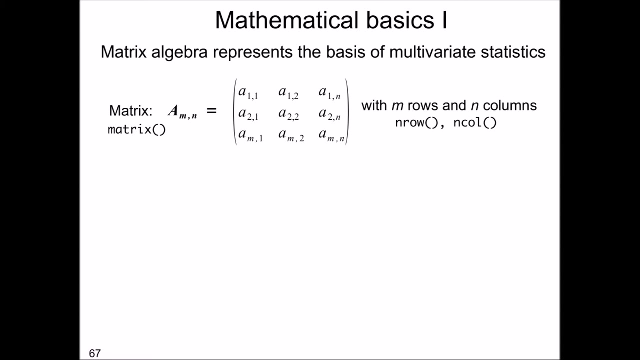 And we checked which variables have the highest explanatory power, assuming that they have a correlation coefficient. And that was the relationship with our endpoint. So we used MRA here for an explanation of observed phenomena in the field. To understand multivariate statistics and MRA. 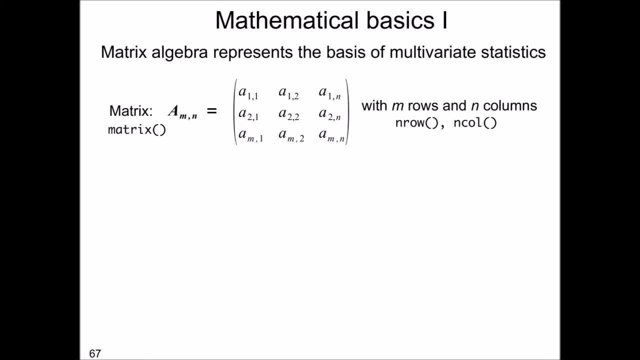 we need the mathematical basis, and this mathematical basis is predominantly matrix algebra. You should know from school that the matrix is given by rows and columns and you have a certain way of denominating rows and columns. First you have the row and the second number gives the column In R you. 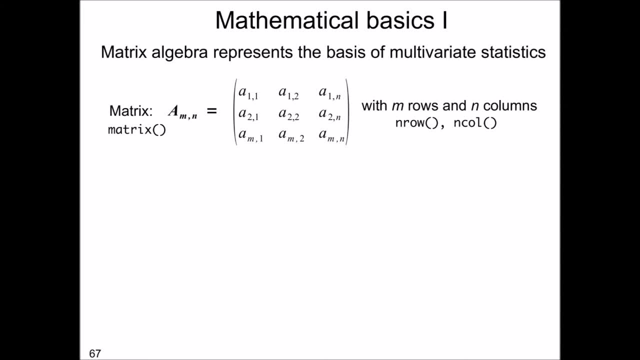 can count the number of rows and columns. with nRow and nCol We can transpose a matrix that's shown here. That's a symbol that you encounter very often. The T means the number of rows and columns, The T means transposed matrix. It's done in T bracket, open, bracket, close, in R and it's 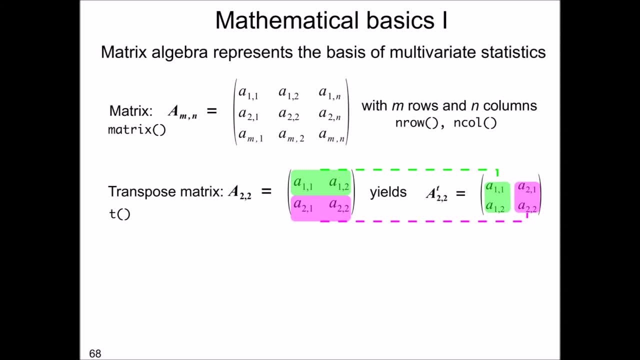 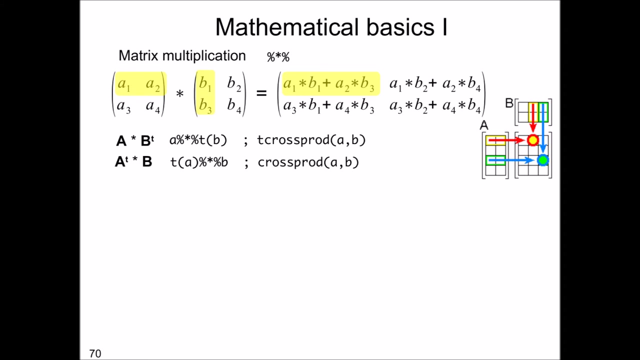 shown here how the resulting matrix looks like. So addition and subtraction of matrices is displayed here. That is not very surprising how this works and you should be familiar with it. Other aspects of matrix multiplication include that you multiply the first row with the column of the second matrix, and you see this here in this little figure. 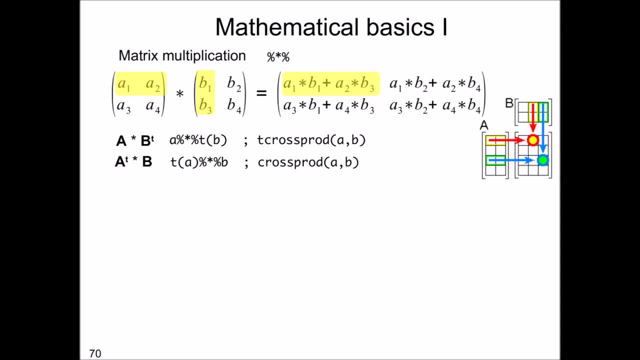 as well on the right side, how this is done, And this is the typical way how matrix multiplication is done, and obviously this cannot be done for any two matrices, but you need to match the number of rows and number of columns between the matrices, The identity matrix. this is a term we should know as well. 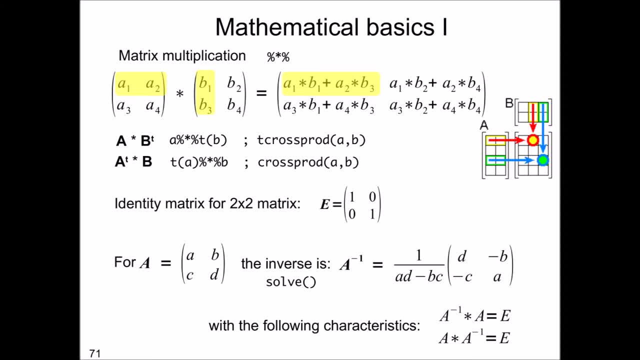 This is a matrix where all numbers, values along the diagonal are one and all other values in the matrix, in this matrix, are zero. And if you multiply the matrix with the identity matrix, you obtain the matrix itself. So the inverse is a matrix which, if you calculate, if you multiply the matrix with the inverse, 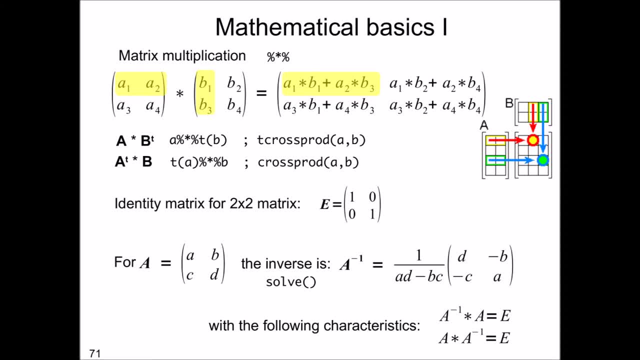 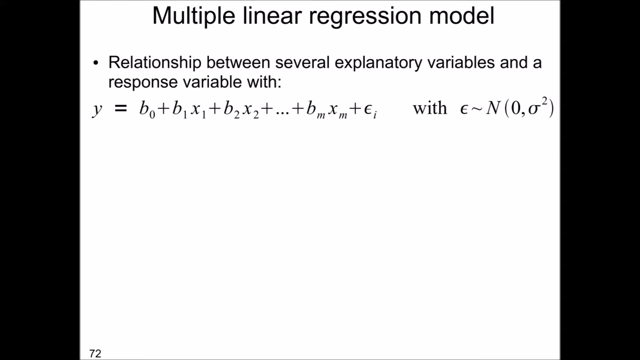 then you obtain the identity matrix. Since we have no division defined in matrix algebra, this can be regarded as something similar as division. So let's go back to the multilinear regression model. Here you see a formula for this model in notation that we use in the course. 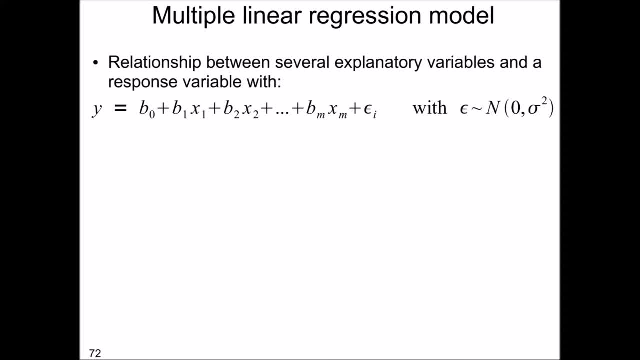 So you have the y- this is the response variable- and you have the betas, which are the regression coefficients that you've already seen for this model, For the univariate, for the b-variate regression model, And we have different x's, and these x1 to xn give the variables, the explanatory variables. 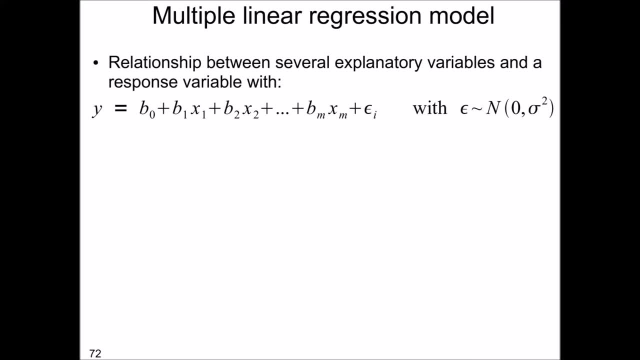 or predictors. So we have an error term and this error term is normally distributed here, in this case with a mean of zero and a variance And a certain variance. The aim is to minimize the error, which is SSE in the linear regression model, And this is given by summing up the squared differences for each value of y, for each observation. 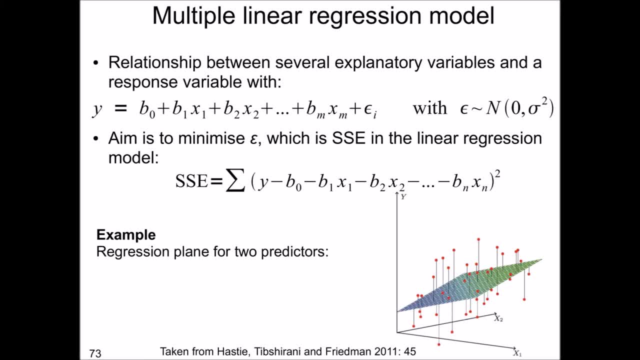 and the related values of the explanatory variables for x. So the result. So the result. The result is a regression plane, This minimized. if you minimize this error, you have an ordinary b-square fit that results from this optimization and you obtain a regression plane here in the case of two predictors. 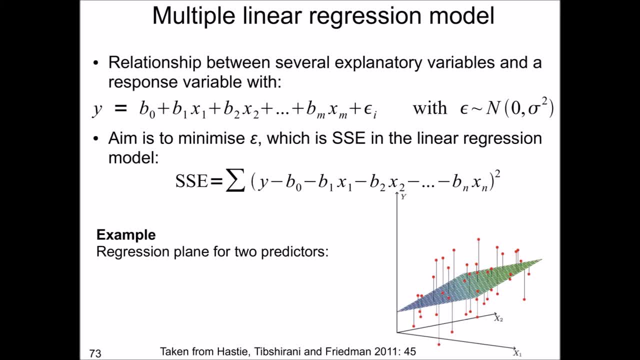 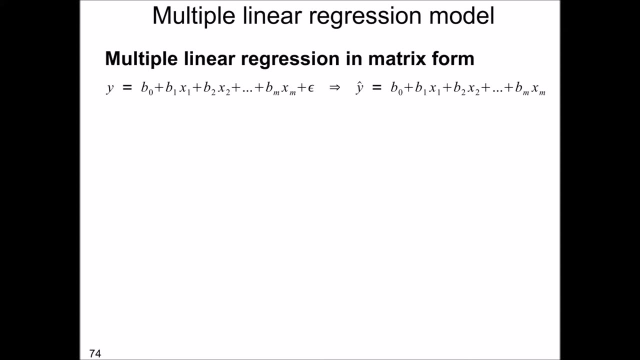 So a plane that is minimizing the distances to the points. You can also express the multiple linear regression equation that has been shown in the previous slide in matrix form, and I will show you how to do this. First, we see on the left hand side the given notation, as before and when we think about 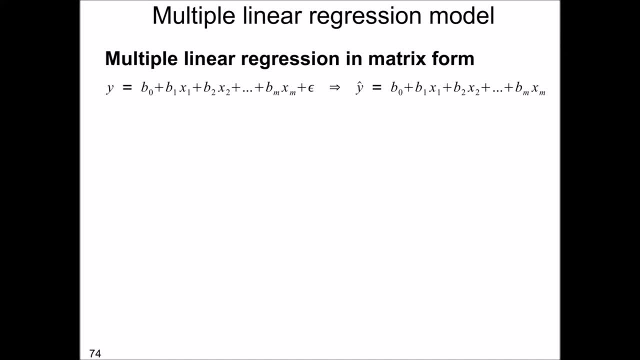 the fitted y. Sorry. So the fitted model with y-head, where y-head is estimated by the betas multiplied with the different explanatory variables, The full notation for each fitted y, So for each y-head, Would be b-zero, Would be b-zero plus b-one, x-one-one, and so on and so on. 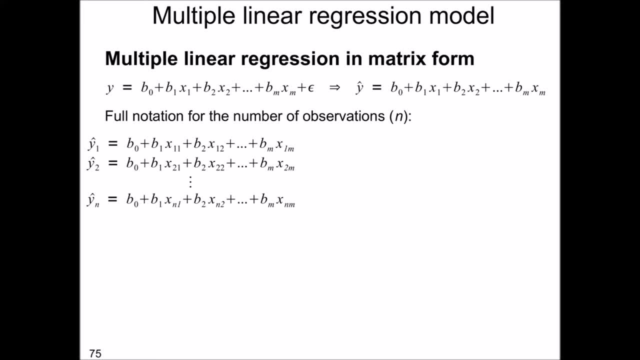 So you see, this is the notation here, And to simplify this kind of notation, instead of having so many equations, we can just write this in matrix form. The matrix would look like this: You have the vector of the fitted y And you have a matrix with ones in the first column for multiplication with the intercept. 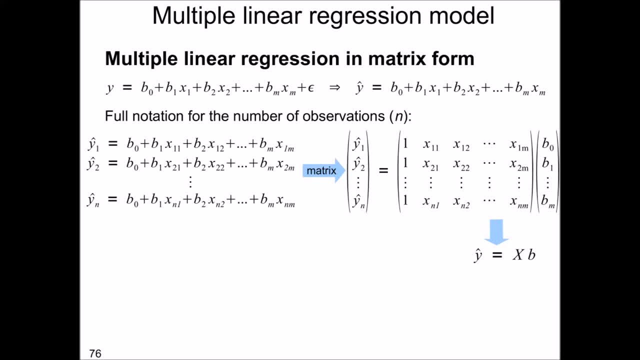 term b-zero And the rest of the matrix is filled with the observations that were made, the explanatory variables And in short form we can just express this as: the vector y-head equals x multiplied b-one- again the beta vector. This should be the beta vector. 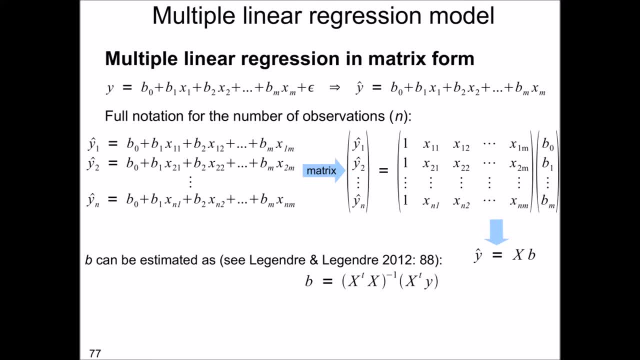 And we can estimate this beta vector from the x matrix, and we see here that to do this you need different operations that we have discussed for in the context of matrix algebra, the basics of matrix computation and, for example, you need to transpose a matrix and you need to calculate. 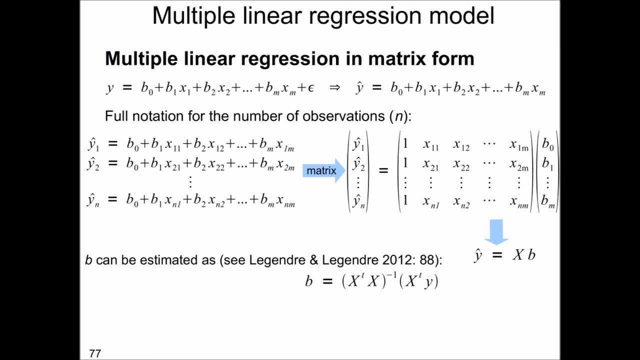 the inverse of a matrix, and these operations are necessary to find the betas. Now we can substitute the beta with the fitted y, So y, hat and x. And if we do this and do some rearrangements- and I'm not going into 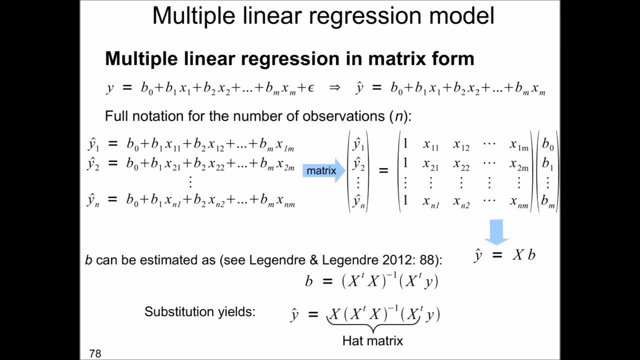 details here because you can look that up: 2012,. then we have an equation where we see, on the left hand side, we have the y hat, the fitted y values, and they result from a multiplication of y with several other values, operations that are done of the matrix of predictors. 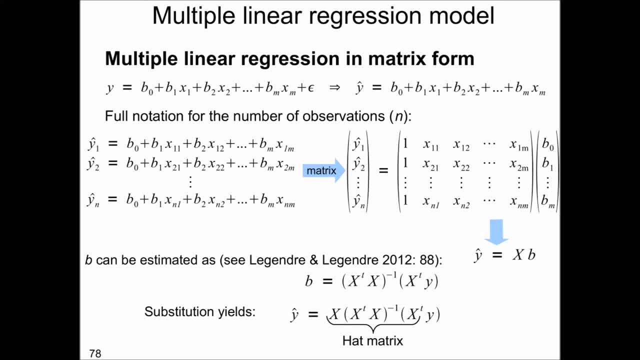 So what basically happens here is that, through some operations of on the predictors and the multiplication, we with y, we have the fitted y, the y hat, and this is called, therefore, these. the matrix that results from this operation of the predictors is called hat matrix, since through multiplication with y, it puts a hat on the y, figuratively speaking. 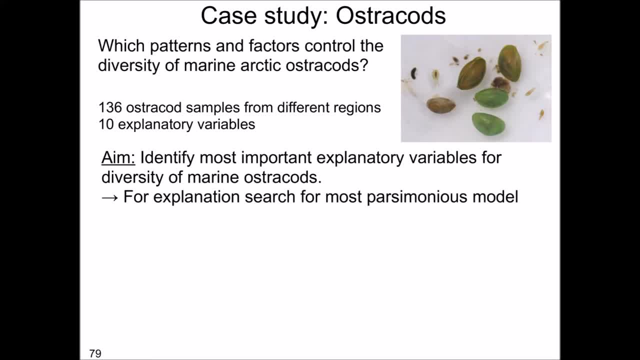 Now in the following, we want to discuss a little bit more for an applied example what multiple linear regression means, and the example that I chose is a case study on Ostrakov. K lives in a very large ocean of a city called K. The fish that that fish visit the ocean comes from Beirut to get food from it and expert 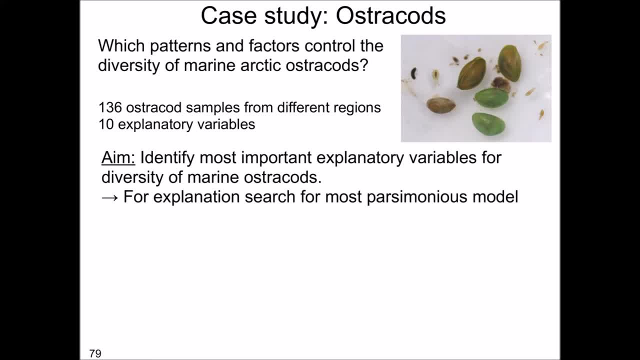 from it comes from Hugo, often happens to live in a tropical subcontinent, which is the region where a ontological structure is located. K has three node union. you have the slice Hemonomic Bent Frontal. you have three individual inch seab opp Somalian observatory. you have two cross로al and live terrestrial aussil. 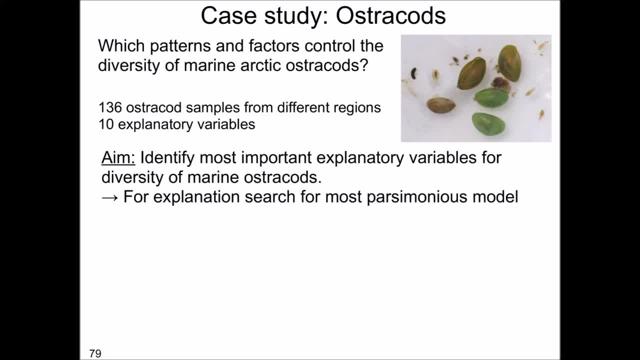 In the four collector sua have twoSuMA in the specialist hospital and the last unit has two electroph graduation and the fourth case study in serftem. So here we have the linear kyrafoeling with u linear regression model. We have 136 ostracode samples from different regions. 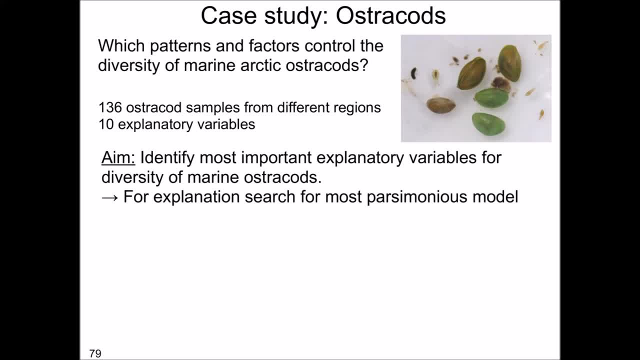 and 10 explanatory variables. We will learn about this case in the practical part, in the implementation with R. So the aim is to identify the most important explanatory variables for the diversity of marine ostracodes And in this sense we search for the most parsimonious model. 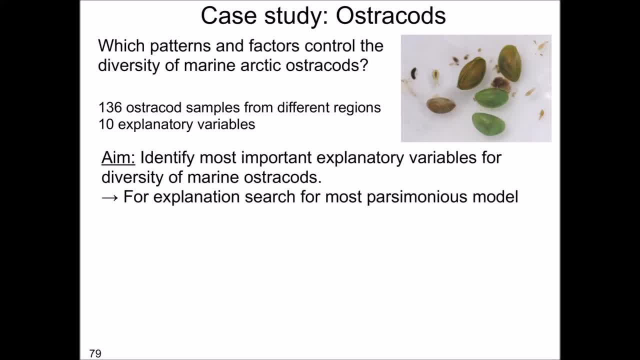 Why do we search for the most parsimonious model? Well, a principle that applies here is the so-called Occam's razor, And this principle reads as follows: It is futile to do with more things that which can be done with fewer. 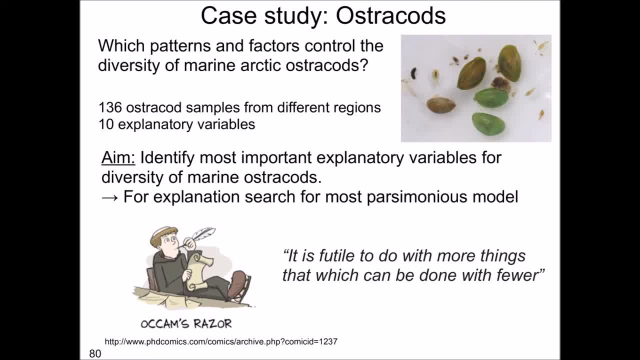 So, translated to our situation, it means, given a similar predictive or explanatory power, models with fewer variables are generally better than those with more variables. If you can explain a phenomenon in nature with one or two processes, why should you use seven or eight processes if you don't achieve more explanatory power? 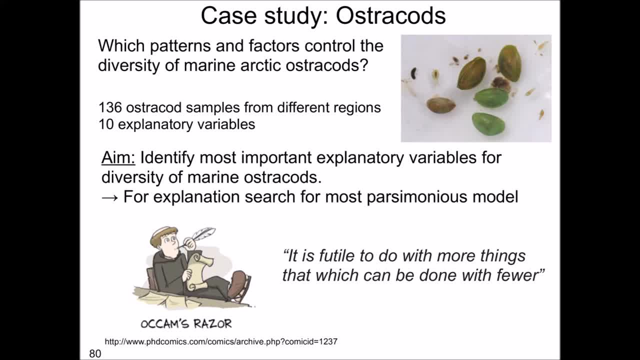 For example- and this is perhaps a little bit ridiculous example, but let's imagine you have an explanation why a clock is ticking: because you have one process. You had a mechanical explanation for this. Now you can add a couple of variables, like: there's a ghost in the clock. 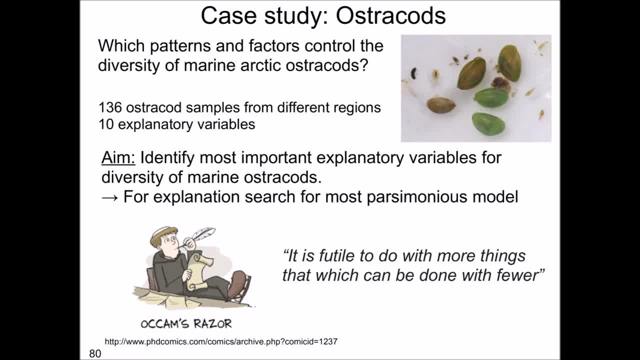 that is, in addition, moving the clock. The clockwork makes the clock move, The clockwork makes the clock move, The clockwork makes the clock move. And you can see. you achieve the same explanatory power by just stating: well, there's a mechanical action. 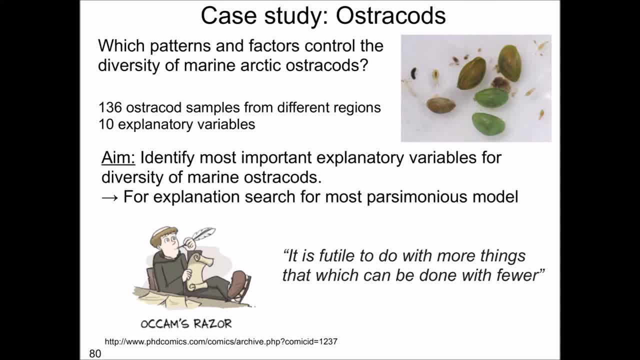 in the clock and the clockwork that makes the clock run. And to add a ghost in the clock doesn't add any explanatory power. So this applies, of course. this parsimonious principle applies when we search for explanation. There's a debate whether, when you want to predict, 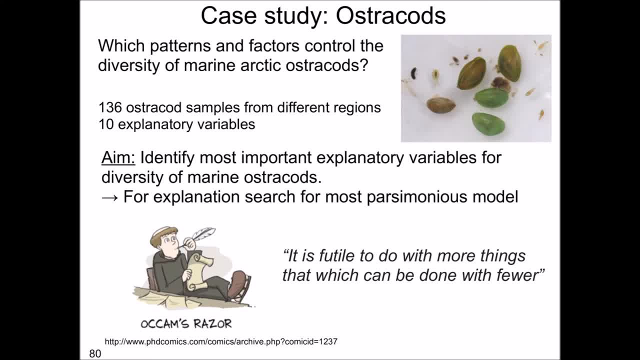 you should just use the full model and include all variables that you have, because this wouldn't harm. Harald suggests that this should be done in Harald 2015.. And nevertheless, I would argue that when you have some variables that make no sense. 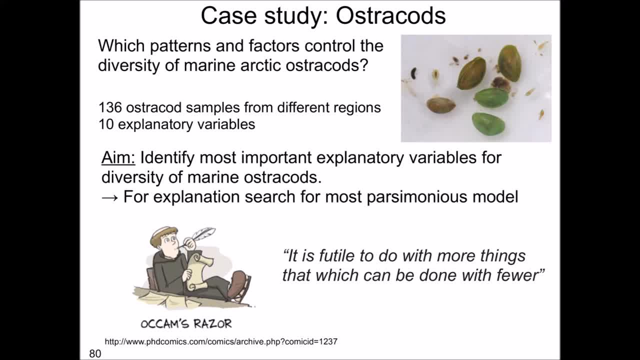 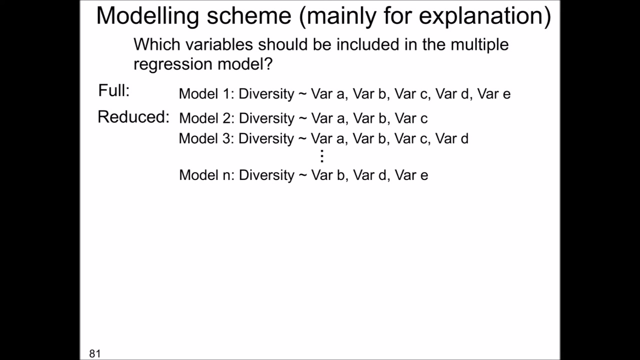 or are known to have no relationship with the response that is to be predicted, I would leave them out of the model if they have no explanatory power. So parsimony applies also to this situation. So how does this modeling work And the scheme that is presented here? 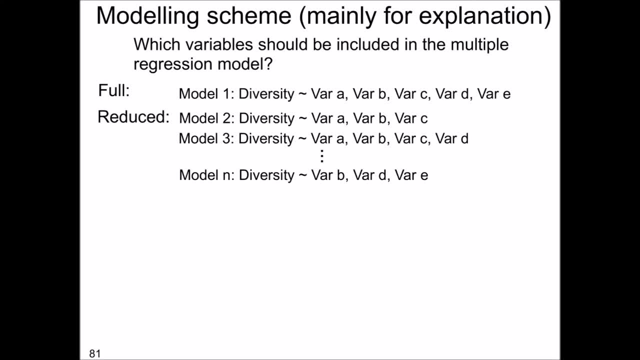 applies mainly for explanation, Not only I will give some remarks, what you would do when you have other aims than explanation in the context of regression modeling. So the question that we posed on the previous slide can be translated to which variables should be included in a multiple regression models. because if we say 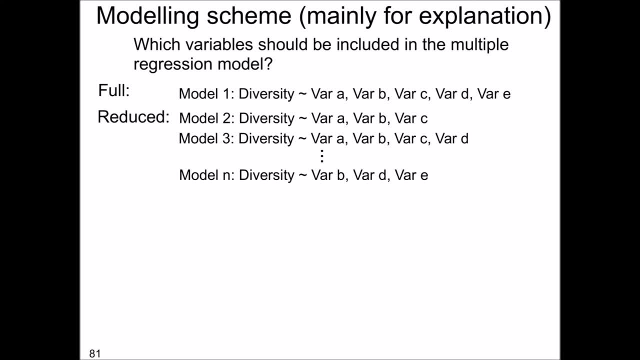 we search for the most parsimonious model. we can construct many different models. we can construct the full model that's indicated here by the first line. that was the model one- diversity, as explained by a couple of variables, and we can have several reduced models where we have only a few variables. 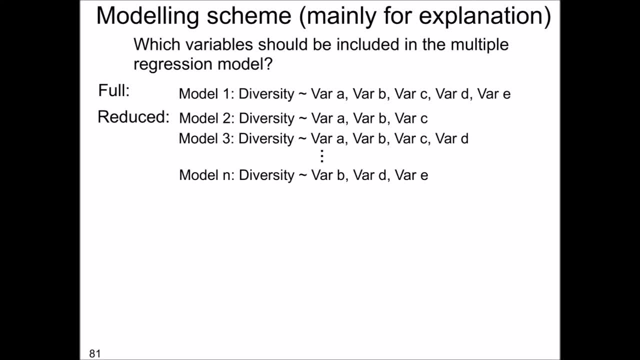 picked and there are many different options for such a reduced model. but how can we decide which variables we should keep in the models, which ones are the important ones? how can we achieve or arrive at this reduced model? well, we could basically just test the important importance of variables using multiple b variate regressions. there's one point that i want to make here. 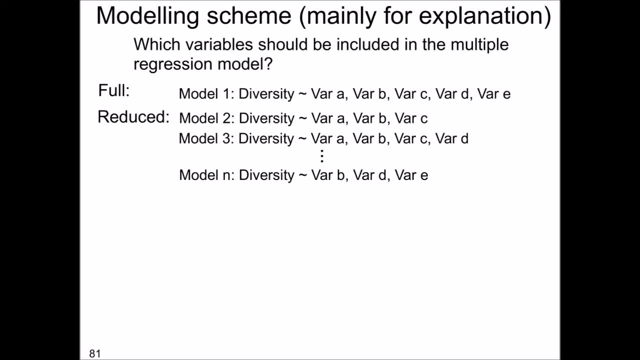 problem here? the first problem is, of course, that if you do many hypothesis tests, then you have an inflation of p values and you run into troubles. but, more importantly, there may be additional variables that exert a high explanatory power, power in the model after other variables have been included in the model, and he would not detect this and think that they are useless. 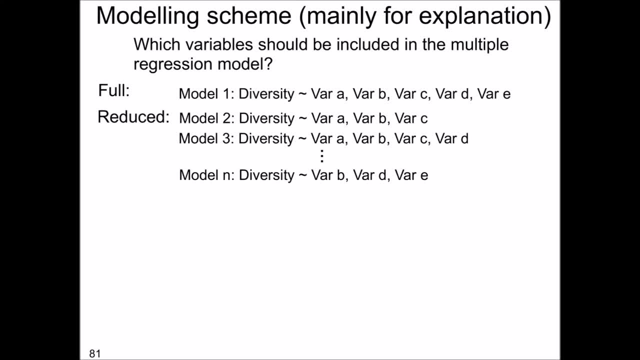 for example, it may be that after correcting or after temperature explains some decomposition of leaf material in streams, that nitrogen may explain remaining variability in the leaf decomposition. but this is also apparent, only apparent, in the situation that you've already explained: the temperature effect. so temperature had been 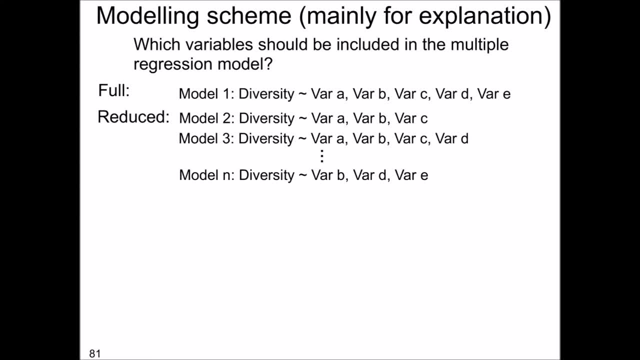 added to the model. so let's look at the strategies that we have in the case of explanation. on the one hand, we could compare pre-specified models or based on scientific knowledge knowledge. we established a couple of models and compare, compare them. then we could have the strategy to to select the best. 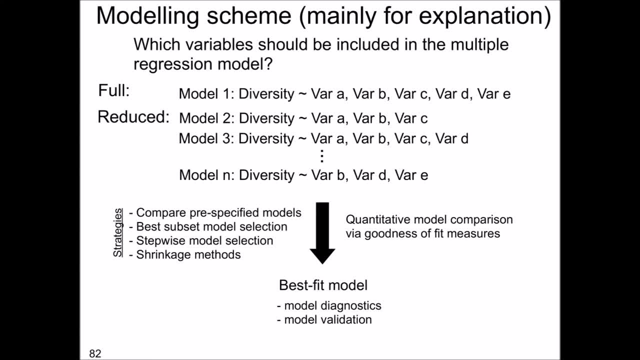 subset models, or we calculate all possible models and select the best subset. we could have a stepwise model selection. so, based on some criteria, remove we will remove, or we add variables to a model, or there are so-called shrinkage methods that i explain later on. so obviously for model comparison, 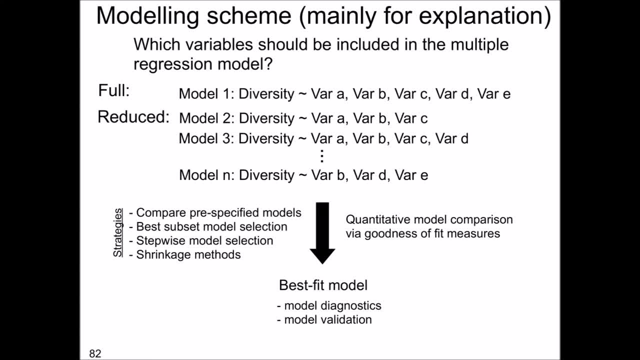 whatever strategy we choose, we need a quantitative, to be able to quantitatively compare the model, and this is done via so-called goodness of fit measures, and by running one of these strategies we end up with the best fit model, and for this we need to conduct model diagnostics and 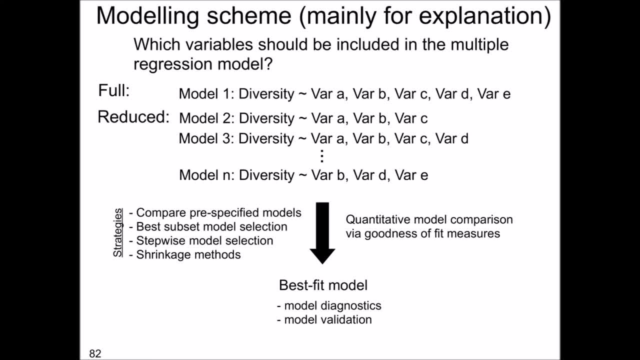 in some cases model validation, unless this has been done before. note that this strategy does not necessarily apply for prediction because, as discussed before, for prediction we may sometimes just we may just keep the full model and do not need to select a modeling strategy. also, if we want to determine an effect size or test a specific hypothesis, we should have a pre-specified model. so 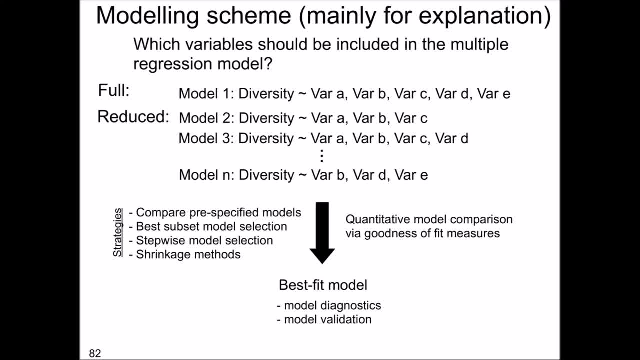 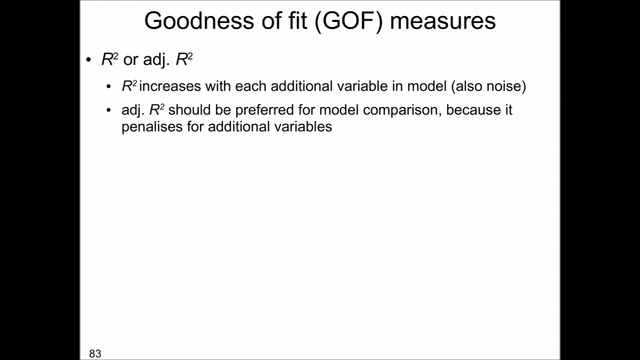 know before what are the hypotheses we want to test and which variables are important, and the same holds for the effect. sizes and the other strategies are more or less relevant in this case different goodness of fit measure, and we will discuss them in the following. we need them to. 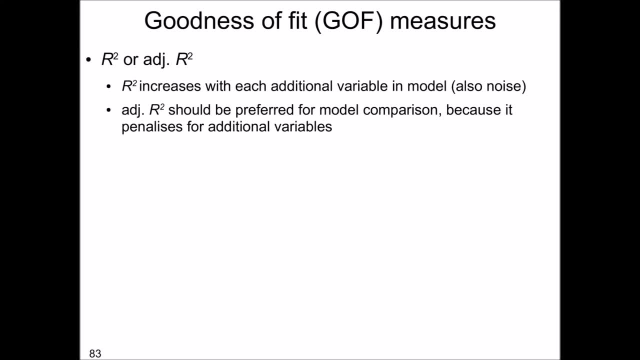 select the model. as mentioned before, one commonly used measure for measuring the goodness of fit that you certainly know is the r square. the r square describes the amount of explained variance in a model, so how much of the variability in the response variable can be explained by your predictors? one problem of the r square is that this automatically increases with each. 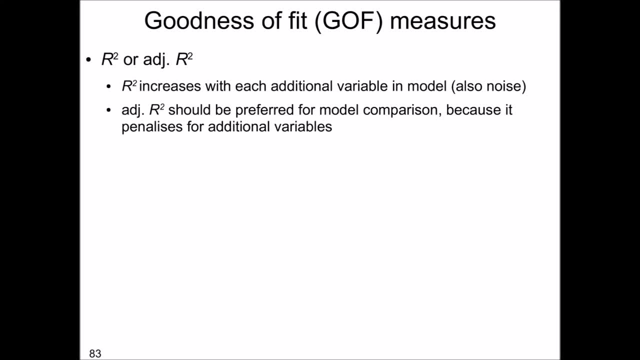 additional variable that you enter in the model. so let's say you add complete random variables that have just been constructed from sampling from a normal distribution or something like that, then this variable would add explanatory power to them to the model in terms of r square. so noise variables are not, are not distinguished by this metric. so 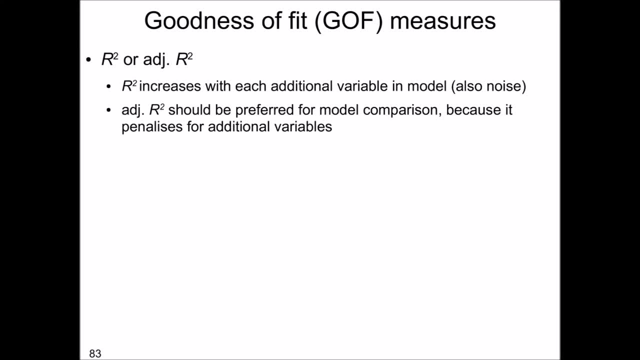 there's no penalty for adding additional variables and every additional variable has a little bit of it explains a little bit of the remaining variance. so if you want to use this measure and you should use the adjusted r square- we have discussed the adjusted r square before. the r square penalizes the model for the number of. 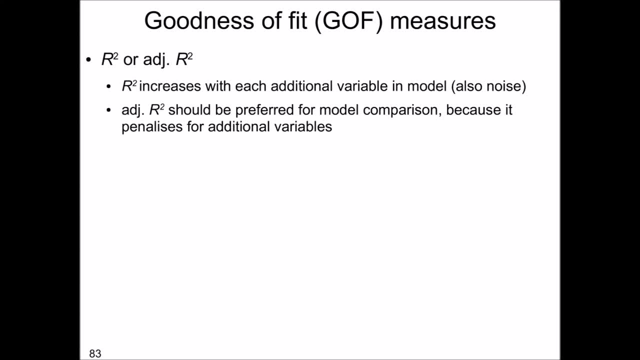 parameters. so that means you have a penalty term. and if you add a noise variable that explains only a marginal, marginal additional amount of explained variance, then the penalty term that you have for entering more variables into the model prohibits that the r, the adjusted r, square, is increased. 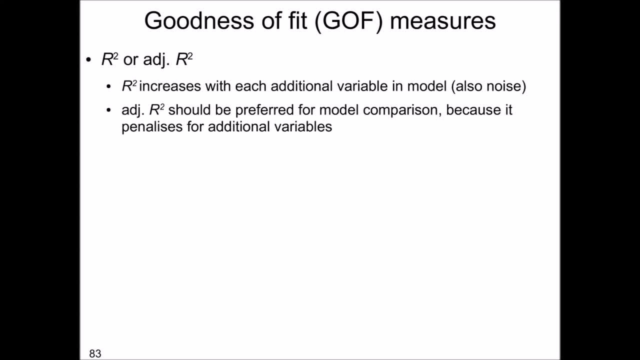 so you should prefer this model. if you target the explained variance, however, the penalty is not really strong by the adjusted r square, and other measures may be more useful. an additional group of goodness of mission measures are the so-called information theoretic goodness of fit measure. they include the aic and the bic. that's the call, that's the akaiki information criterion. 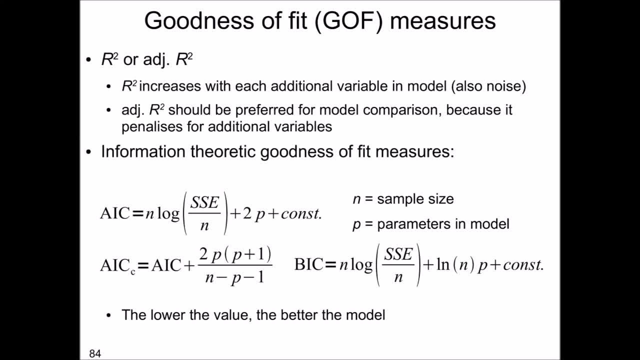 and the bayesian information criterion and they include also penalty terms and the sample size for measuring, the goodness of fits. so you see, in the formula for the aic you have the sum of squared, the sum of squares related to the model, the error sum of squares divided by the sample size. 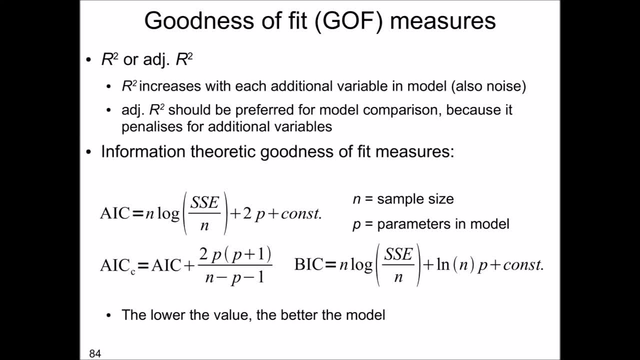 and there is an additional penalty term that includes the parameters and the constant. we are not going into details here. however, if you think a little bit what this means, this means that the more parameters you have in the model, the larger the AIC becomes and, at the same time, the more the more error sense, unexplained variance you have in. 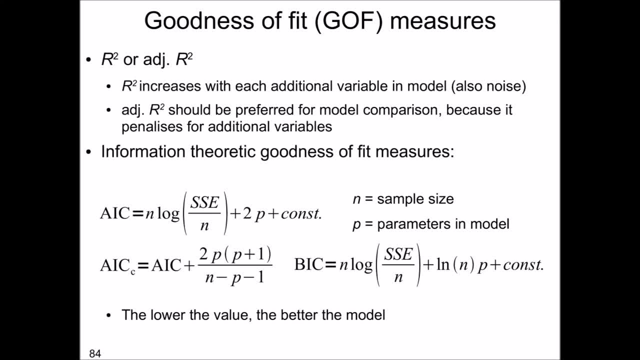 the model, the higher the AIC becomes. now, if you add noise variables, you have the same phenomenon as for the adjusted R-square. you may reduce the unexplained variance or the error sum of squares a little bit, but you get penalized by this additional parameter in the model. 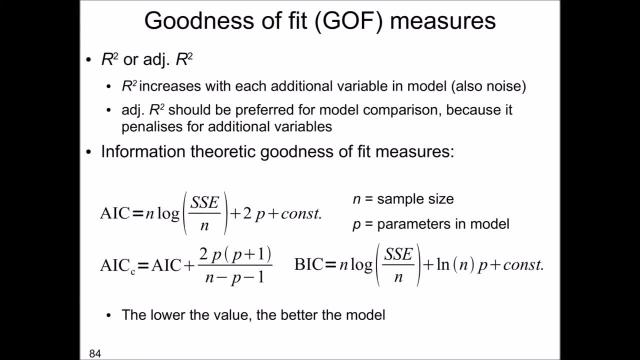 and you see, the main difference between the AIC and BIC is actually that, instead of AIC having two times the parameter as penalty, you have the logarithm of the sample size as multiplier to the number of parameters for the BIC. This means generally, the BIC is more restrictive when it comes to entering 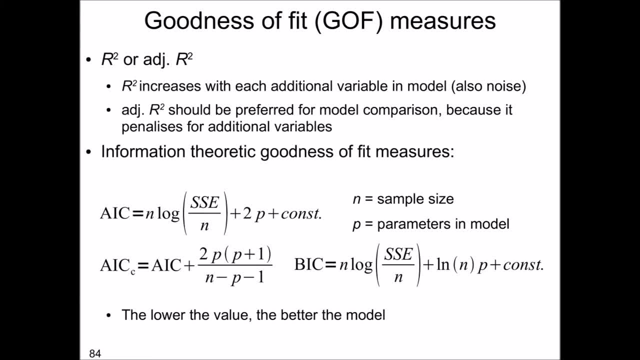 variables into the model. So if you want to search for the most parsimonious model, then you would generally tend to using the BIC. Now we haven't really discussed yet how we decide which model is better, and one strategy is for the AIC or BIC to just use: choose the model with the smallest AIC or the smallest BIC. Other strategies: 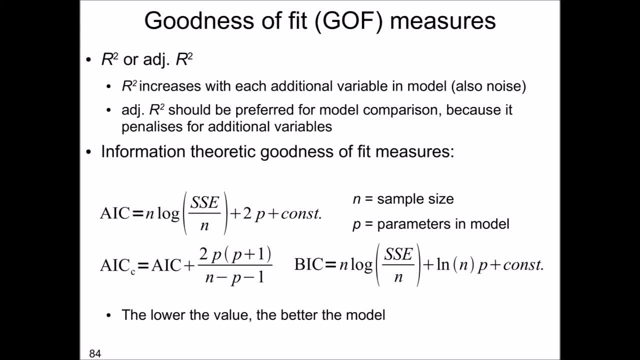 but include to choose all models that have a lower AIC. So you set a threshold and you consider all models that fall within certain distance to the lowest AIC and then you could average them. I show you how this can be done in the R-Script, although i'm not really in favor of averaging models and 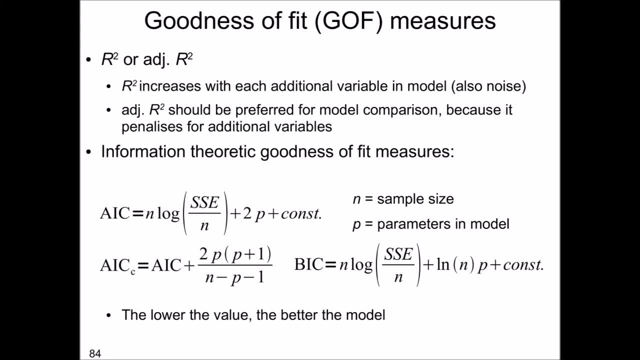 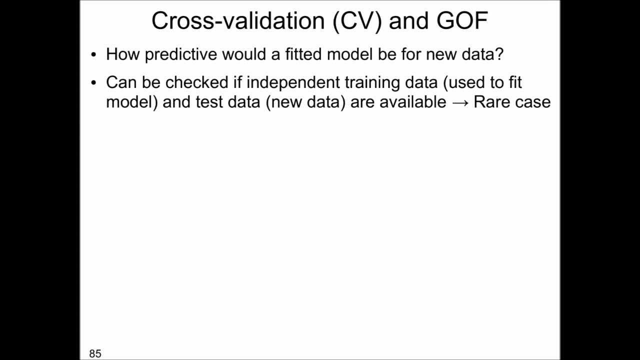 more about this in the next part. Thank you. Another approach for selecting the best fit model is called cross-validation. It's typically applied in a different context, namely to validate the model after it has been fitted, but it can also be used as a cross-validation for the BIC model. The BIC model can also be used as a cross-validation for the model after it has been fitted, but it can also be used 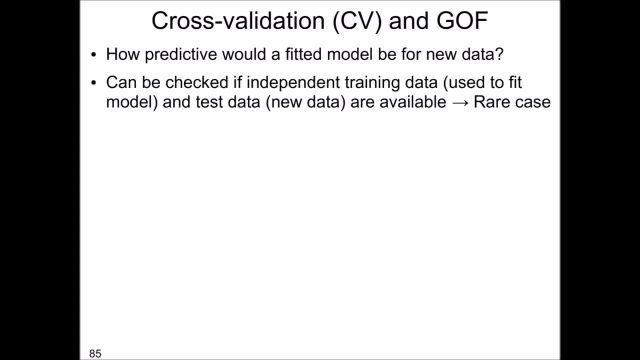 for selecting the best fit model And it's driven by the question: how predictive would a fitted model be for new date? This can be checked if you have independent training data and test data. So let's say you have a data set which you use to fit the model and another data 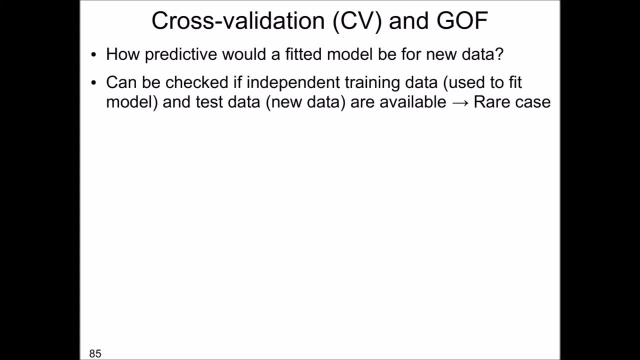 set which you use to test the model. For example, you have monitored some environmental variables and you predict the species richness in one area, and then you go to a completely different region and you check whether your model applies there as well, which means you can use your environmental variables to again predict the species richness. 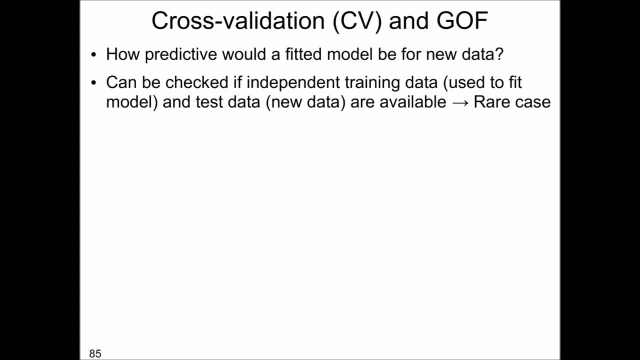 However, one problem is certainly that we don't usually don't have independent data. Most data are generally based on data from a specific research question. if you don't have independent data set, then you can't really apply this strategy, So one possibility is to use your existing data. 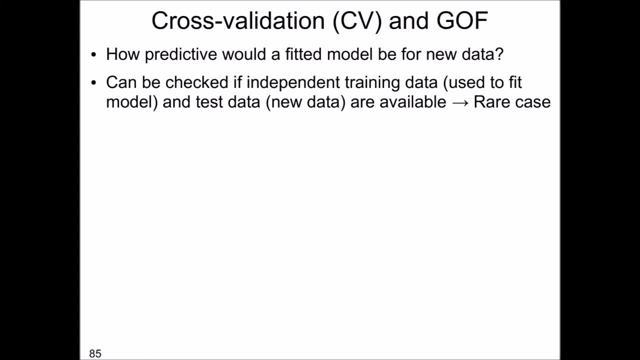 and separate this into different cases, And this can be done with cross-validation. So cross-validation randomly divides your available data in a training set and a test set and does this randomly a couple of times and then predicts the known observations in the test set and you can see how much your 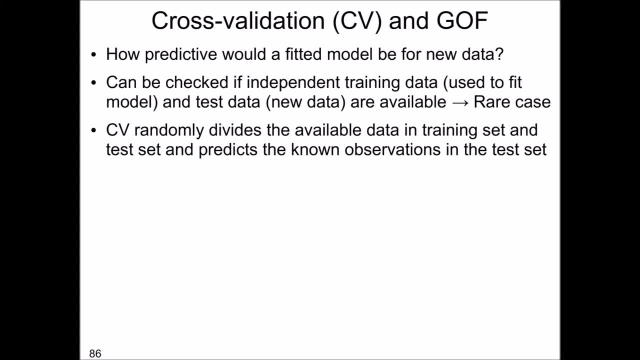 predictions deviate from the values of these observations. In this figure you see a display how cross-validation works. there are different kinds of cross-validation. cross-validation here is displayed on this figure, the so called five-fold cross-validation, so generally K-fold, which means you split the data into five random samples and through 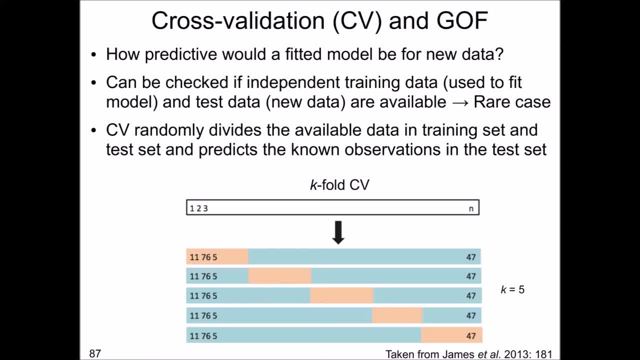 each Okay into. through each iteration you choose the remaining 80 percent of the data to predict. this removed 20 percent of the data and then you average across a predictive power for these five fold cross validation. typically, five fold or tenfold cross cross validation is used another. 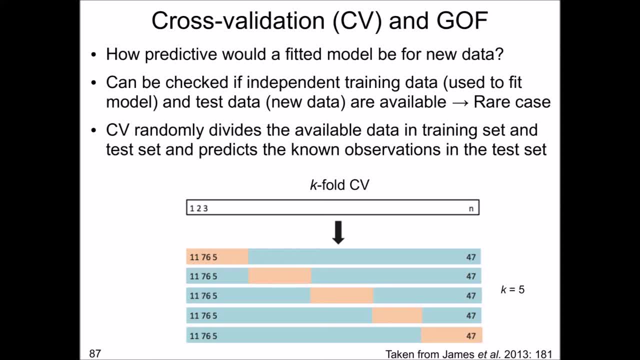 possibility is to use leave one out cross validation, which means that the model is fitted n times, where n is the sample size that you have, and each time you remove one of the observations and you use all other data to fit the model and predict this removed observation, however, 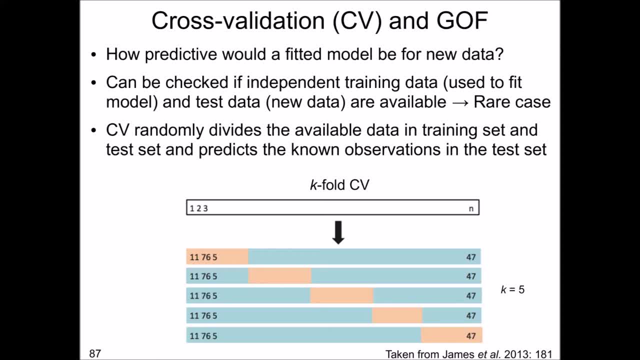 you can clearly see that if you have a relatively homogeneous data set, then removal of one of the observations does not lead to much, does not lead to a good assessment of the prediction accuracy. so generally, five or tenfold cross validation is more recommendable anywhere any. any way, you have to consider that when you 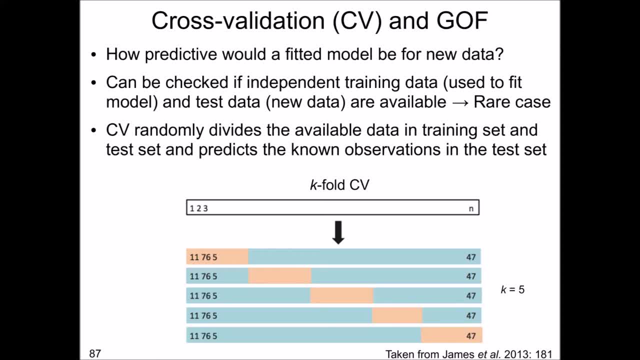 have this data set from one region, for example, that for the example that i gave before you, even if you remove parts of the data, this still underestimates the general prediction accuracy for a completely new data set of a different region or something, or from a different time. 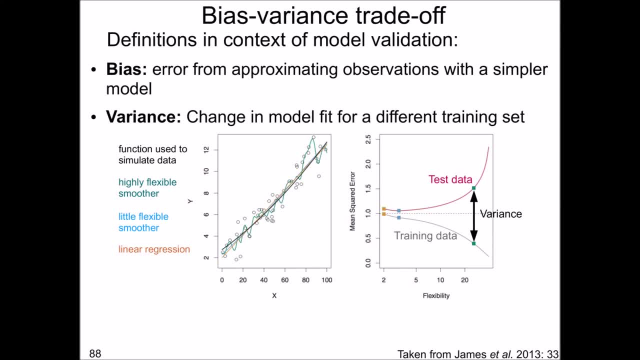 there is one issue that we have to discuss in the context of model selection, model validation, and that's the so-called bias, variance, trade-off, and this is best understood by looking at to the figures that i display on this slide. so, first of all, when we discuss the 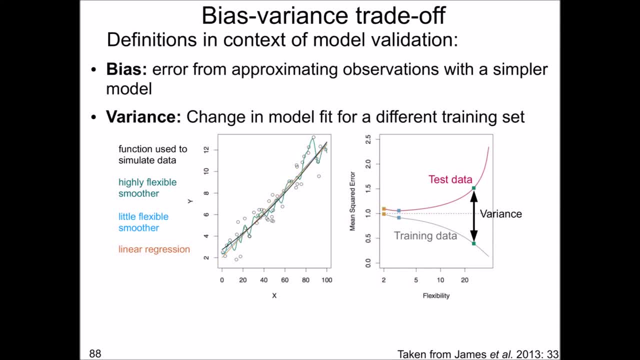 base by variance trade-off. we first have to to discuss what bias and variance mean. bias means it's the error from approximating observations with a simpler model. so we always do statistical modeling. we have some simplification. that's one general, generally model. we cannot include all processes that drive a. 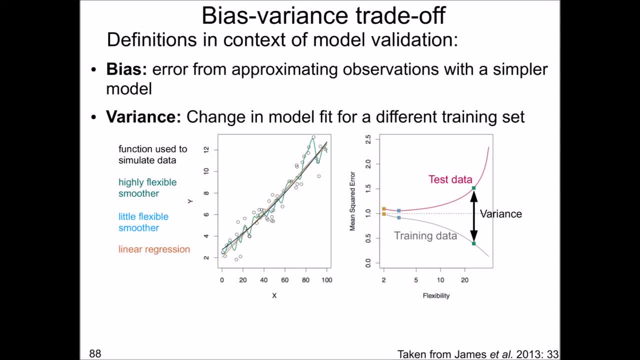 phenomenon. we focus on the most important ones and generally, and that is why we have remaining error in our data and we have variance. that is the change in the model fit for a different training set. so if we use completely new data, then our model fit would change and there's the so-called 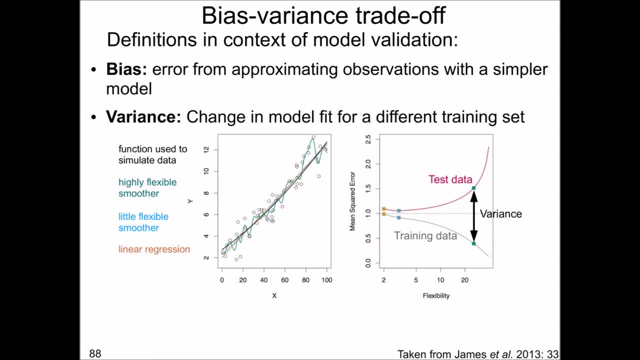 bias, variance trade-off. this means if we have a very, very low error by because we approximate our observations really good, so we use a more complex model and we use, we choose this model to have a low bias, then our variance will probably be relatively high because we have a model that fits our data reasonably. 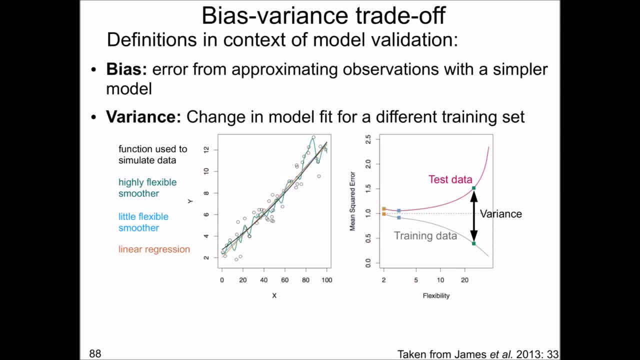 well for the first data set, but any, any data set has its particularities, so it doesn't fit very well to the different data set. so how is this? this shown in the graphs. you see on the left figure we see three lines and one line that follows the points. 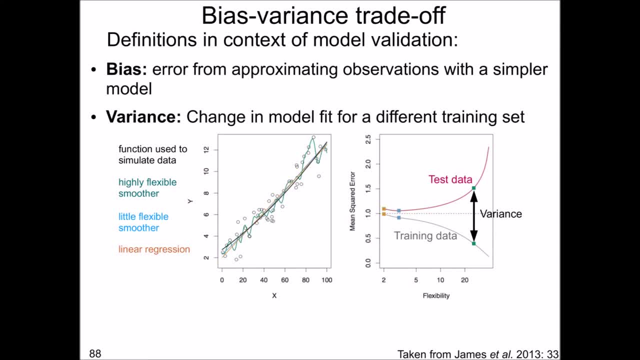 the black line displays the function that has been used to simulate data. this data is given by the points around the line. then we have a highly flexible, smoother, so relatively complex model, a very flexible model and this very complex model that contains a lot of terms to smooth, to capture the deviation of the points from from the line. 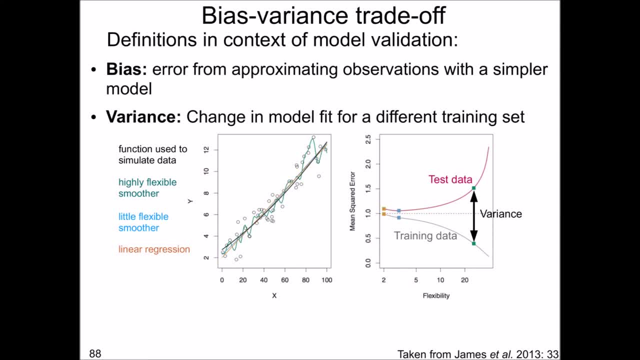 and has a, so approximates this, this, this pattern of the points, relatively well, is is the green line and we have a blue line that has more as a higher error term because it does not approximate the points that well, and we have a linear regression line as well. so we see, in terms 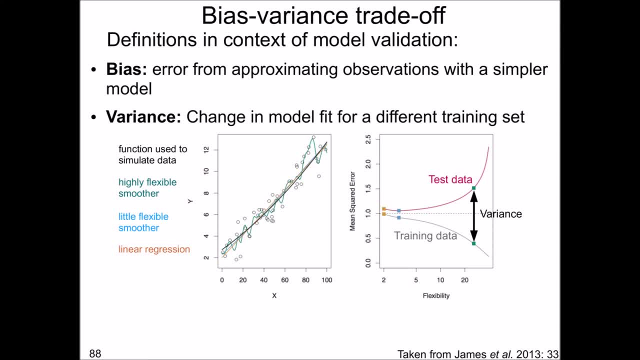 of flexibility, linear regression and the little flexible smoother are. both have a relatively low complexity and a low flexibility and they have a relatively high error compared to the smoother. the smoother is really flexible, so it follows, it approximates exactly the pattern but has therefore has therefore a relatively low error or a low bias. however, if we now choose a different data set, 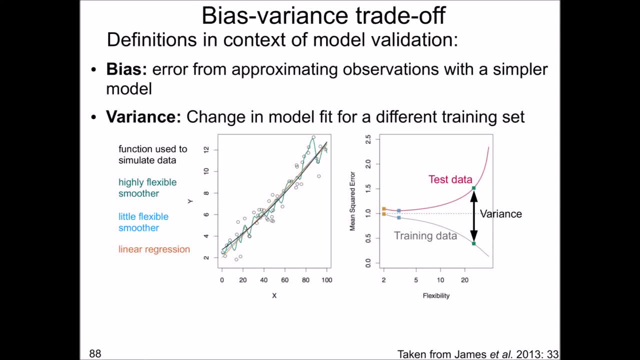 which we want to predict from our relationships that we have established with these models. this is shown on the right hand side. then we see for the brown, blue and green situation that our mean squared error is relatively high for the linear regression. so that's a relatively high bias. but 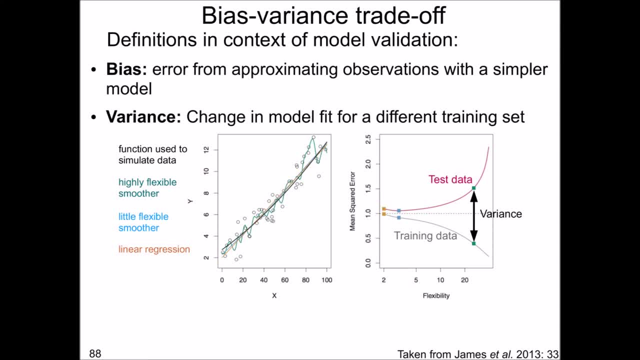 when we predict a new data set, the test data, then we have not much variance. so for both data sets or for new data sets, we have a similar prediction power. for the little flexible, smoother, we have a reduced bias and a little bit higher variance, and we see what is meant if we choose the highly flexible, smoother. 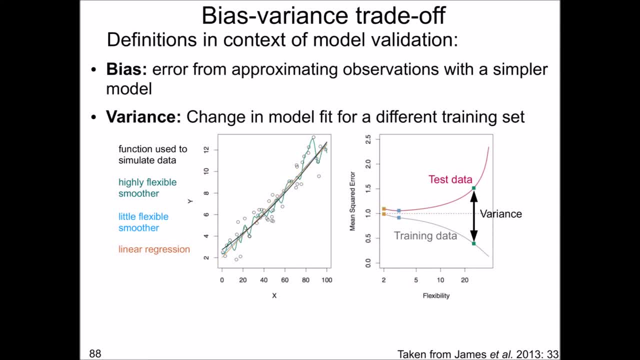 we have a relatively low error for our training data, but if we take a new test data sets, then the variance becomes really high. so we generally can say here that based on this example, we can say that we have a trade-off between bias and variance and we have to decide. 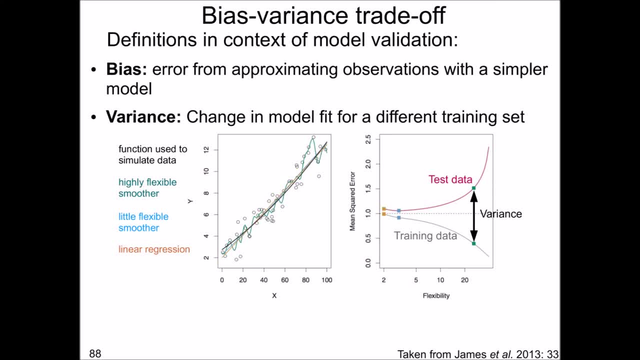 do we want to fit our data really, really well but sacrifice the predictive power, or do we choose a relative variance, simply model that has a low flexibility and has a similar predictive power for both data sets? typically, the bias decreases and variance increases when model flexibility increases, and this is what we have already discussed. 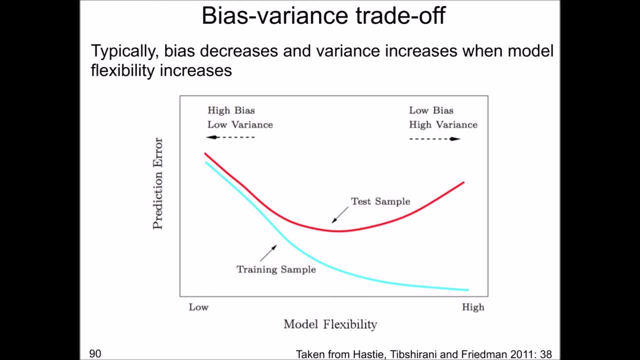 and here is another generalized description of what we have already discussed: if we have a model with low flexibility, then we have a relatively high error, high also so-called high bias, but the low variance. and on the other hand, if we have a very complex model, then we have a high flexibility and 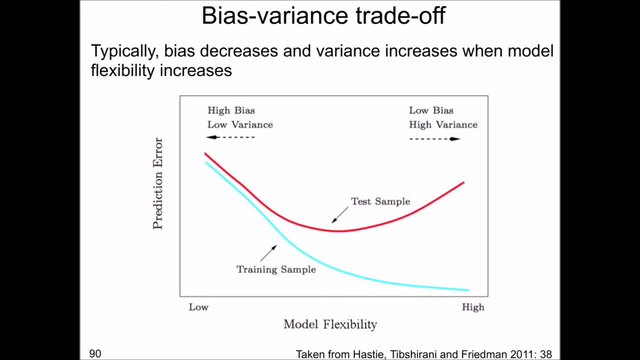 and the low bias, but presumably a high variance. When we optimize identification of a model, we could, for example, search for the position on this graph where the bias, the squared bias, the error and the squared variance from the error when choosing a new model, in sum, are minimized. 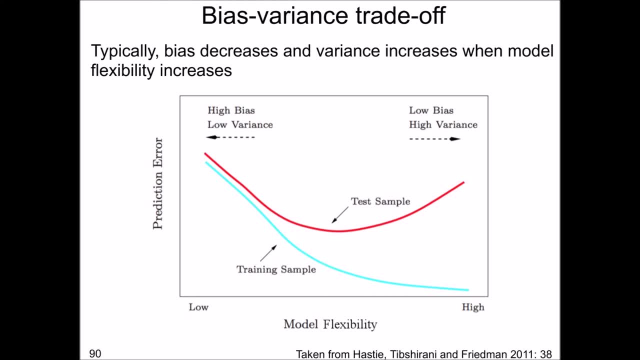 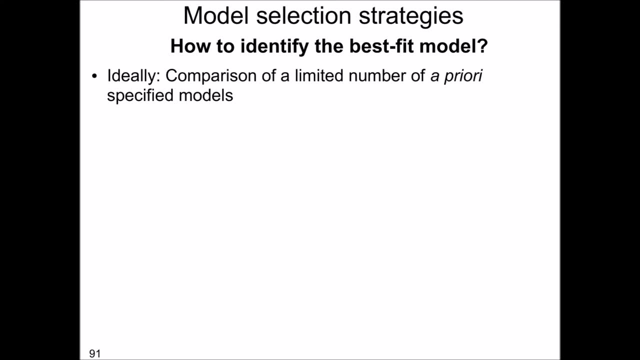 So this would be a strategy. So we have already discussed that there are different strategy to identify the best fit model And we now go more into depth into this: model selection strategies. Ideally we would compare the limit, model limit number of a priori specified model. 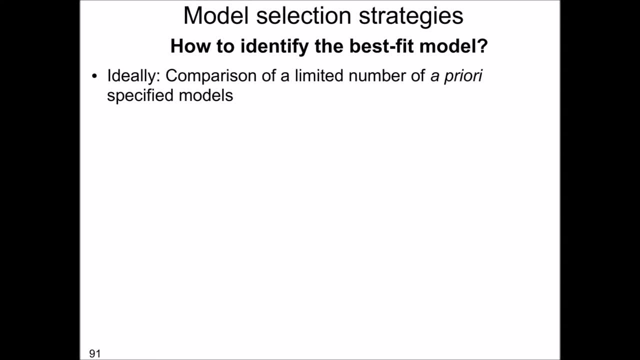 So we know we have a specific scientific phenomenon and we know that a couple of variables may explain this phenomenon and we decide which variables we include And we established, let's say, three, four different models and test Which one of the models has higher prediction accuracy. 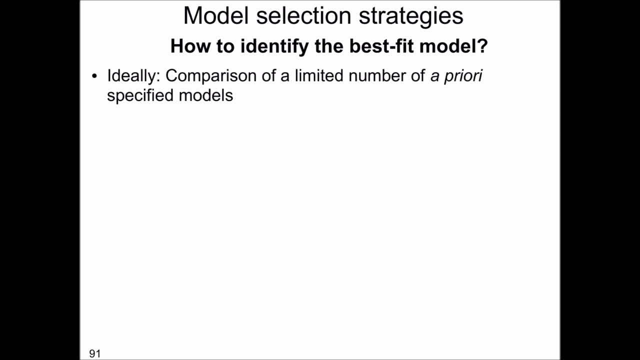 or has a higher explanatory power. Now, often we have the situation and have we have many variables which might be relevant and we don't know exactly which ones of these is not relevant for the first time phenomenon that we want to explain, or when we want to predict. 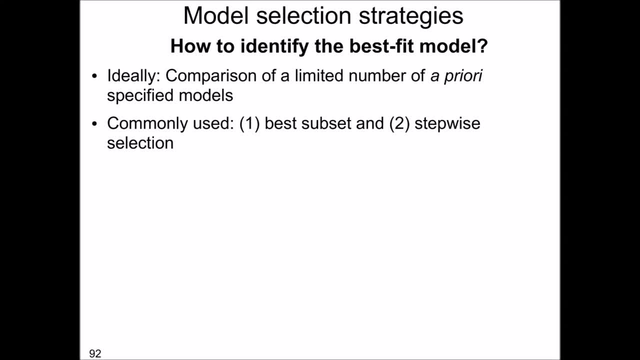 So what is currently commonly used is best substance and stepwise model selection. Best subsets means that we compute all possible models, and stepwise selection means that we look at pre-specified goodness of fit measures for each step of modeling and we remove or add additional variables. 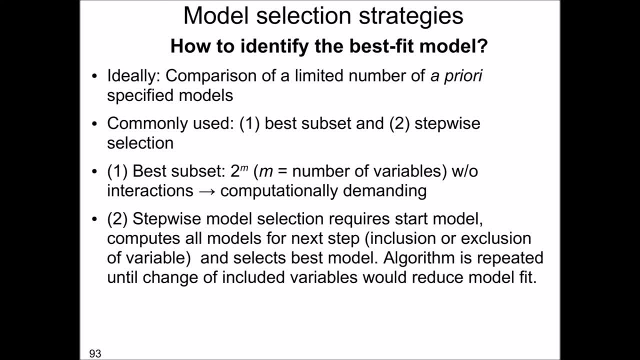 The problem of best subsets selection is that this is a strategy that is computationally really demanding. So, when we have more than 10 variables, compute the computation of all possible models and select the ones that has the highest, for example, explained variance, or the lowest information criterion. 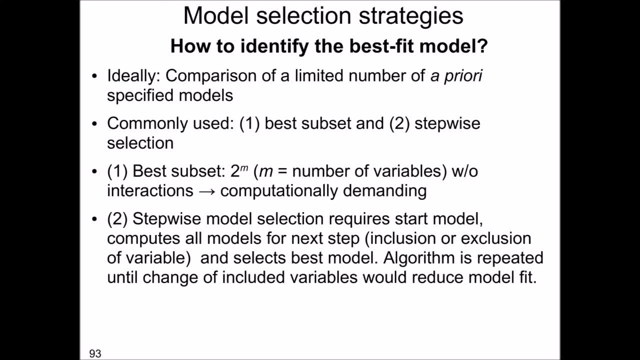 becomes infeasible. This procedure should only be used when we have really no initial hypotheses on the ranking of the scientific relevance of the variables. So let's say we have explored something in space, in outer space, and we haven't been there before. 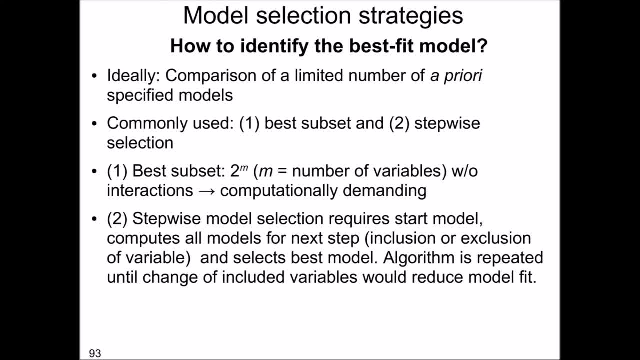 We have many variables that may explain, for example, some occurrence of new life forms on the planet, and we have many, many variables that could explain this and we have absolutely no idea than best subsets. This is something that may be applicable, But typically we have many hypotheses and many previous studies in our research field. 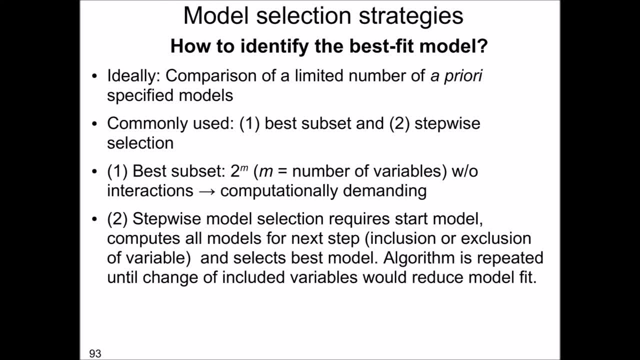 and we can use DEAM to guide us in variable pre-selection and not just calculate all possible models. In addition, best subsets selection also suffers from the flaws that we will specifically discuss in the stepwise for the stepwise selection procedure. So we can't just calculate all possible models. 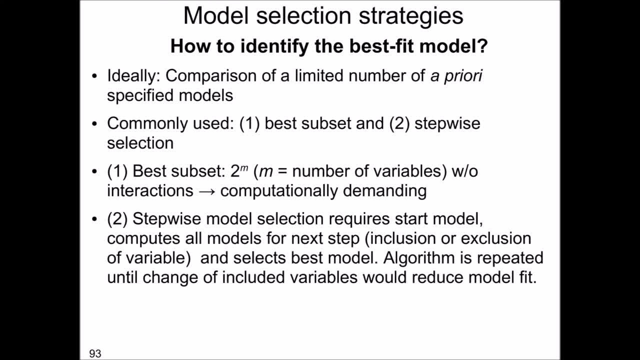 We can't just declare what is the best subsets, So we can't just say that we have a very good result which is much more commonly used. I already have mentioned average model selection, averaging as well, and I give on the slides below. you'll find a really good article that presents some of the 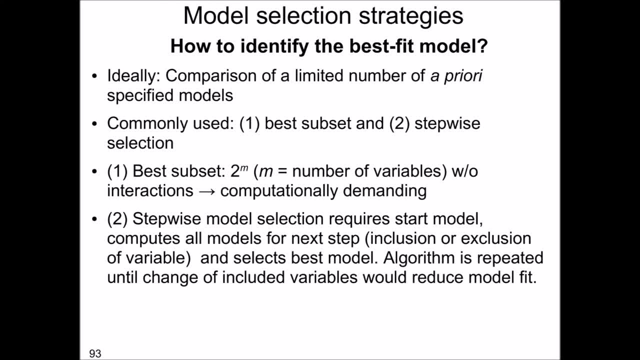 criticism on model averaging that is worth reading. Stepwise model selection functions as follows: You start with a start model that could be a null model- that means the model containing no variable- or a full model- that means the model that can contain that model that contains all relevant variables or an intermediate model of these, and then you 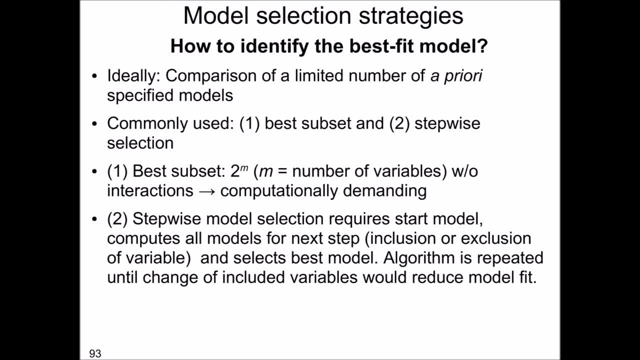 calculate the goodness of fit measure and based on this goodness of fit measure you would decide whether you add a variable or you delete a variable from the model. So you calculate all possible steps that can be taken from the next iterations. of example, if you have 10 variables in the model, you calculate about goodness of fit measure. 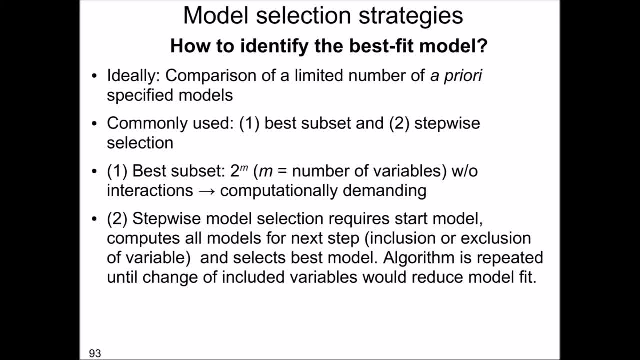 If you remove each one of these variables and then you decide what is the best solution And you repeat this algorithm until the change in the included variables would reduce the model fit based on your goodness of fit measure, though. let's say, when you would have five variables. 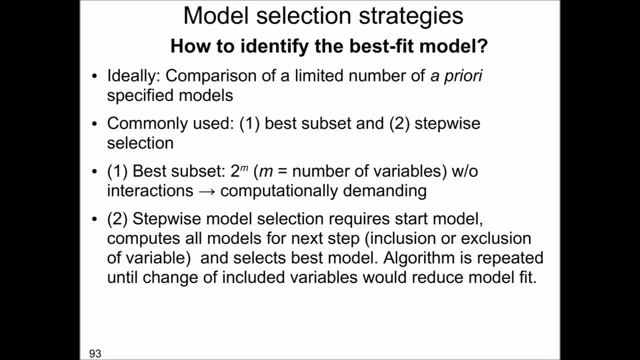 in the model and you would reduce, or the reduction or inclusion of additional variables would reduce the goodness of fit. then you know that this is the solution, stopping point. We don't continue modeling anymore. The following step wards selection procedures are available You can use. 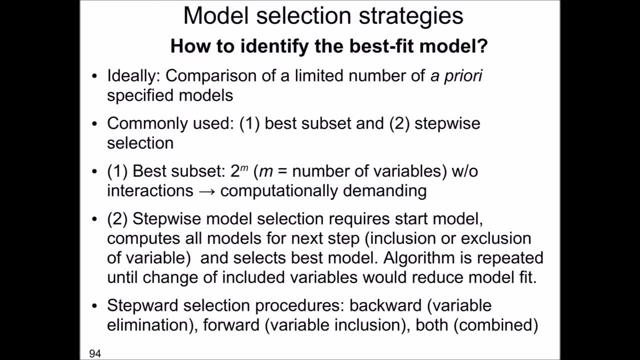 backward selection. It means you eliminate variables from the model. You start with a full model or another model and the only way to the only one. in each step it is checked which variable should be removed or whether this algorithm should be stopped. Conversely, forward step wards model selection checks if an 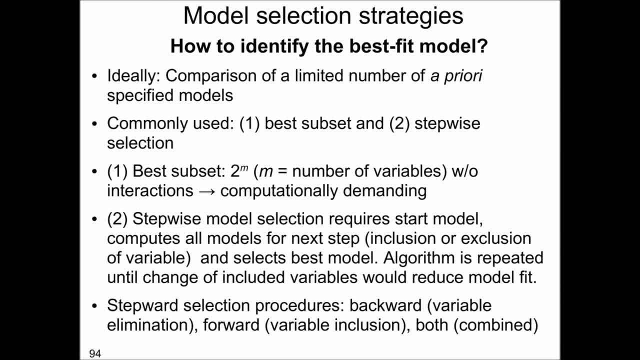 additional variable that is entered increases the model goodness of fit. or you have the strategy forward and backward model selection, which means that at each steps it is checked whether one of the variables should be removed or one of or an additional variable should be included, and based on. 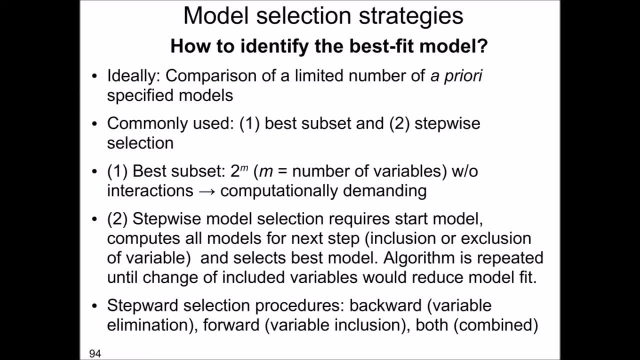 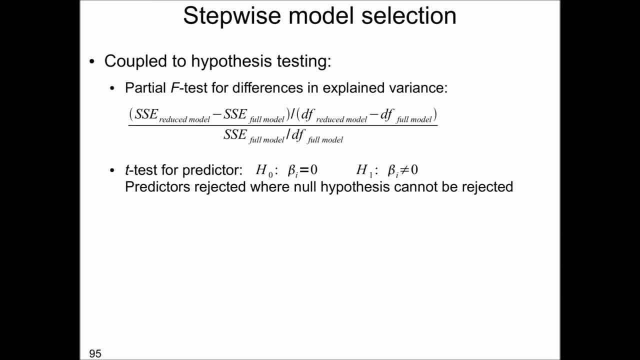 the goodness of fit. for each individual case, it is decided whether the algorithm is stopped or whether another variable is entered or removed from the model. Which goodness of fit can be used? We've already discussed these. On the one hand, you can use hypothesis testing. 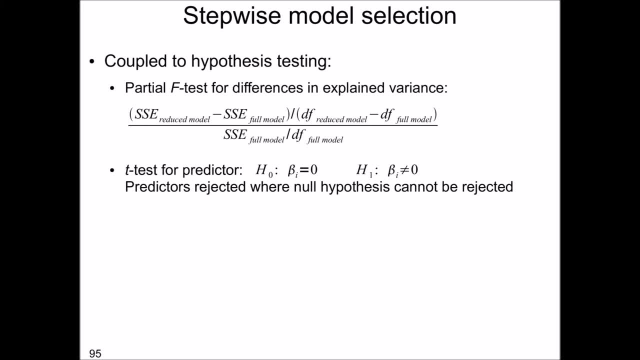 and one test that you have already encountered before in the context of ANOVA is the F-test. Here we use a partial F-test that checks the tests for significant differences in explained variance. You see in the formula The error sum of squares of the reduced model minus the error sum of squares of 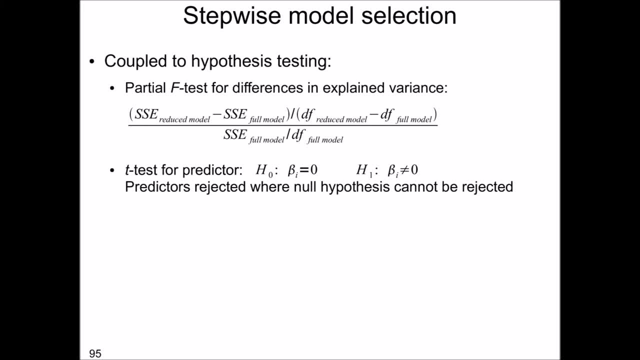 the full model and you divide this by the decrease of freedom of the reduced to the full model. So what you basically check here, whether this drop or a change in the variance is statistically significant, taking into account the change in the decrease of freedom. So for only adding or removing a couple of variables from the model to be, 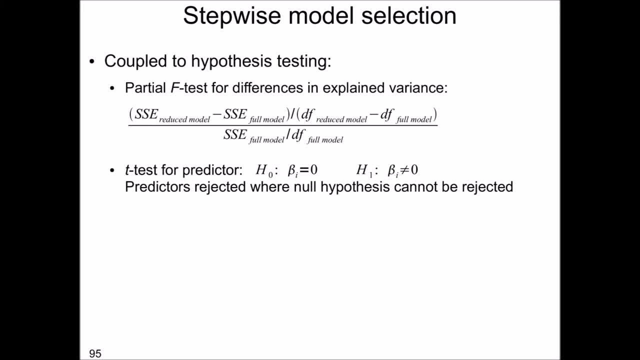 significant, you would test whether the explained variance changes. So if the explained variance doesn't change significantly or considerably, then this test tells us that we can do this because we have the same explanatory power as before. So we basically remove variables or add variables as long as we have no. 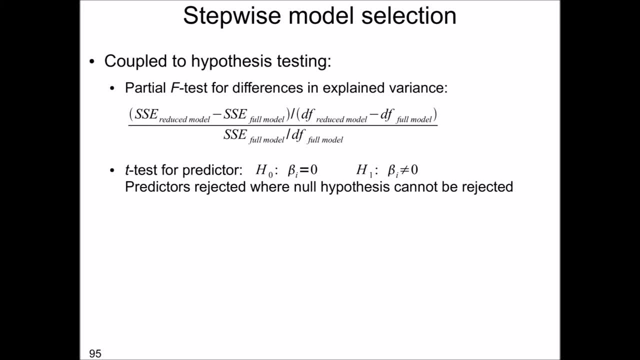 statistically significant differences between the models in the case of removing variables or we enter variables as long as we have a statistically significant increase in the variance. We can also test the predictors in the regression model. for example, we would test here- This is outlined with a t-test- whether the regression coefficient for a predictor is. 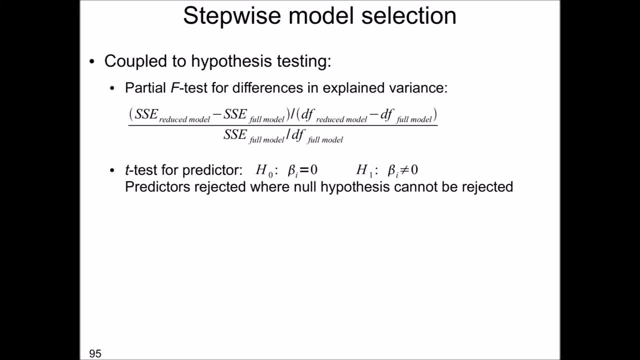 zero with the alternative hypothesis that the regression coefficient is different from zero. So, as you know- you know they have already discussed t-tests in the lecture- when we can write reject the null hypothesis that the beta is zero, then we include a variable in the model, because if the regression coefficient is zero, yeah, then we don't need a variable. 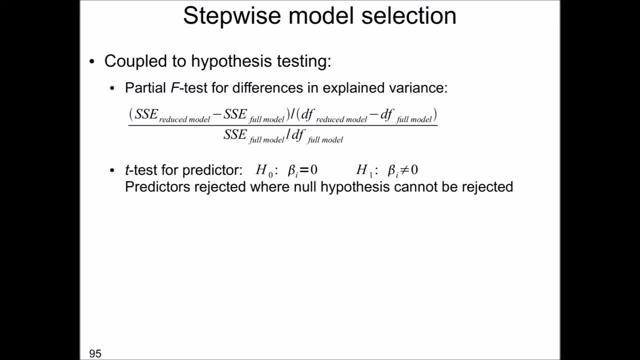 because zero times the values of the variable always are zero, so we don't need to include this variable in the model. There are certain problems that are coupled to hypothesis testing, and one problem is very obvious. you have heard this before. What you do is, if you do a stepwise model selection and you run multiple hypothesis, 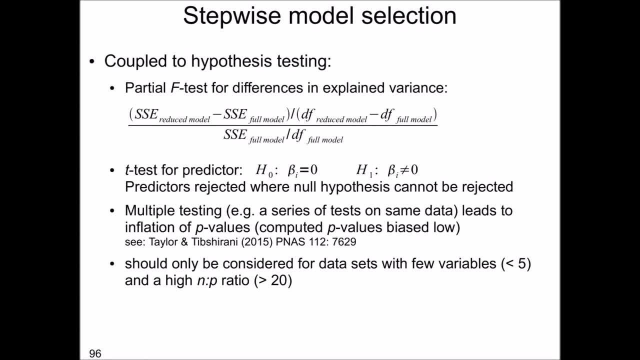 tests that you have an inflation of the piece. That is one of the most common reason: that the rate of change for the increase in the expression of the value of the t-test is two to three times greater than the rate of change of the t-test. so there is a possibility that if the t-test is complete, the t-test will. 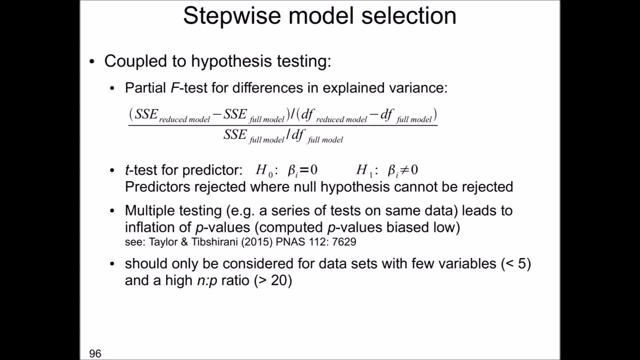 be the result of a process and you may actually get the result in the next lecture, And this is also a really good example. Here we have a harmonic expression of the t-test overestimated, but i will discuss this later in more detail, later on. so if you choose this, 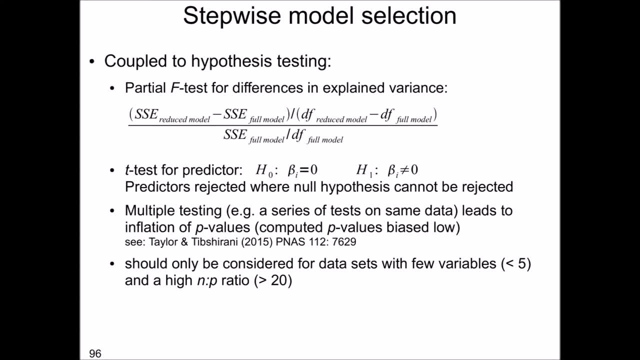 strategy. i would argue that you should only do this if you have very, very few variables, for example small, less than five, and you have a high ratio between sample size and parameters in the model, for example, larger than 20. so if you have five variables, you would need about 100 or 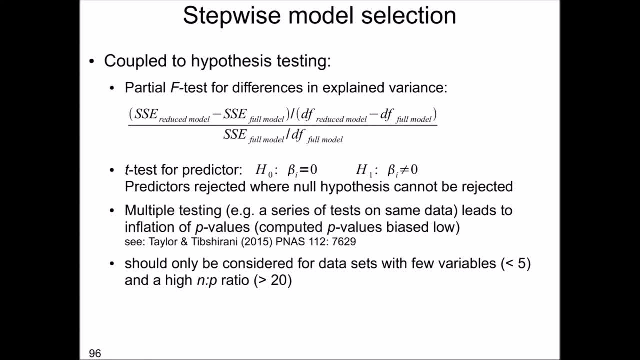 even more cases. to not run into problems with this strategy, a different approach that you can use are information theoretic criteria. so you would calculate the aic or bic at each step when you remove or enter a variable or decide, and then certainly as such, as i discussed before, 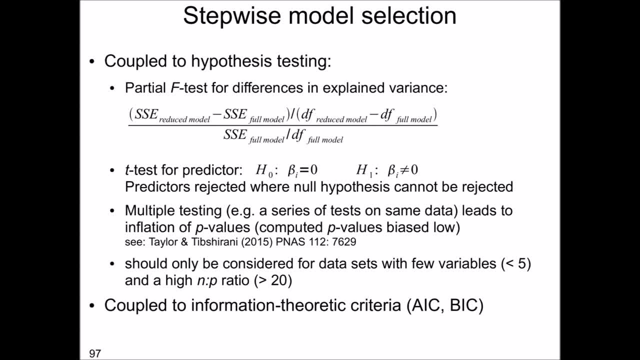 you decide on your primary dato attributes and then you can see that there are many different each step, whether how the AIC changes when you enter or remove a variable and you select the optimal AIC value, the model that belongs to the optimal AIC value. 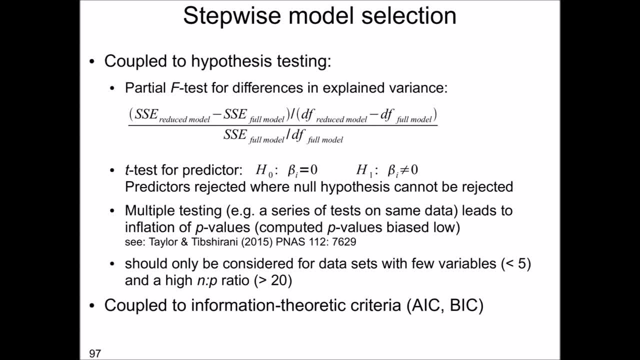 There has been a long discussion whether you should use hypothesis testing and some people argue that information theoretic criteria should mostly be used and are more reliable. however, in the recent publication, Virto showed that actually all these approaches- hypothesis testing based on p-values, but also information theoretic- witness of fit. 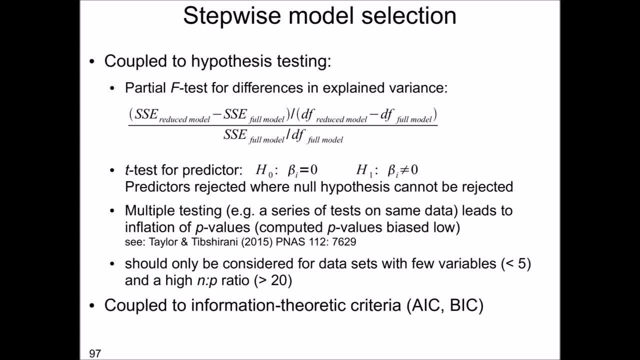 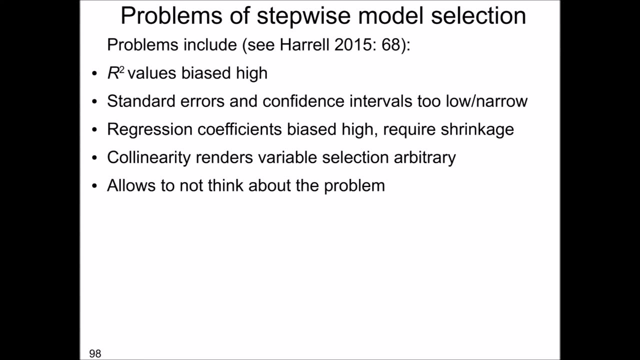 measure are intimately linked, so they basically face the same problems as discussed before. So what are these problems of stepwise model selection? I've already touched upon these and we will deal now with these in more detail. First of all, one problem is that the r-square 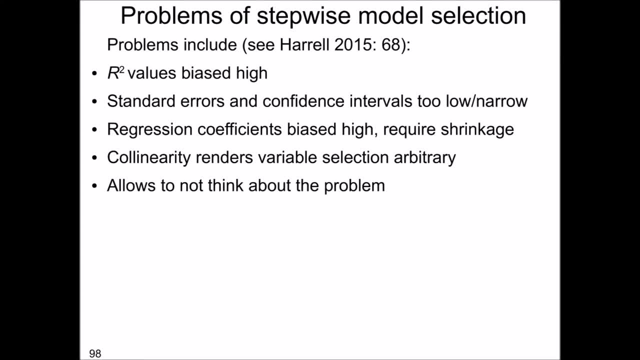 values are biased high, so the amount of explained variance is overestimated. when you do stepwise model selection, Conversely, standard errors and confidence intervals for individual variables are too low, confidence intervals too narrow, so you underestimate the uncertainty that is related to the predictors or in the model. 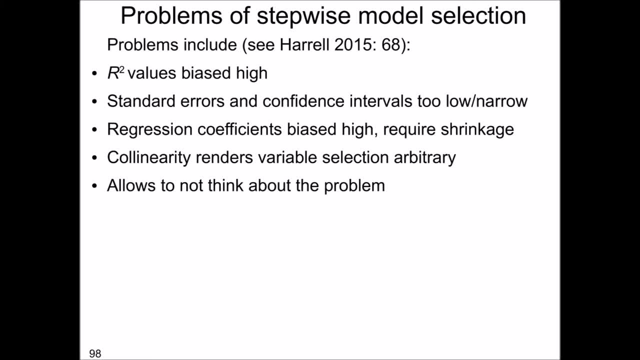 Conversely, the regression coefficients are biased high. so you have for a single case: when you fit a model, then you find the most extreme variables that have an effect, and so the regression coefficients are biased high. and if you would run the model on new data you would almost 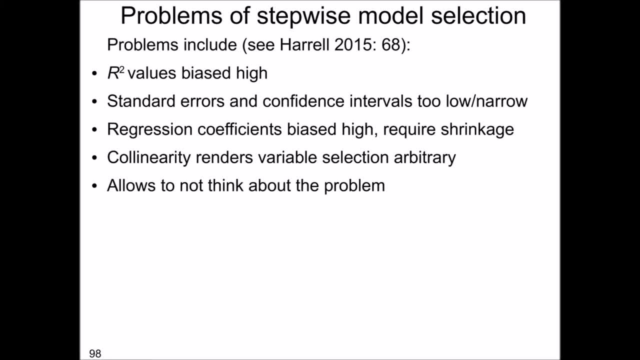 find for the largest regression coefficients that they are reduced for the new data set. But you have, since you have a selection, focus here on you and finding the variable is the strongest effect. Another problem is that in the case of polarity the variable selection is rather arbitrary. 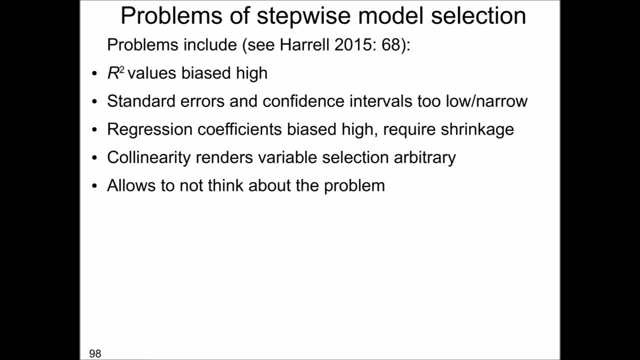 and since we can just run automated procedures- and Harrell, for example, criticized- but others have done this as well- that this stepwise model selection procedure allows us to not think about the problem. For example, even if you know anything about the data, you can just run. 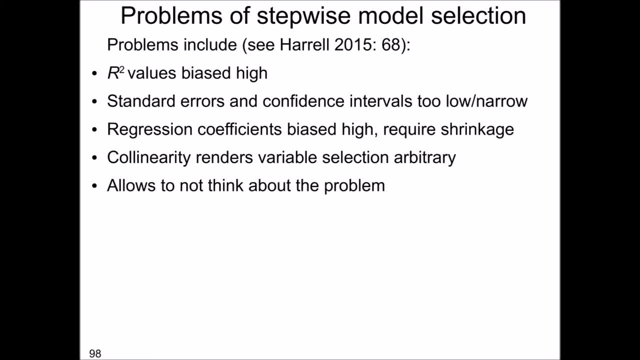 model selection and you obtain a result. Yeah, as I already mentioned, the problems generally apply to stepwise modeling strategy, irrespective of which goodness or fit measure you use. If you have to use stepwise model selection, then Harrell suggests to use backward selection because this performs generally better in the presence of collinear variable. and this starts. 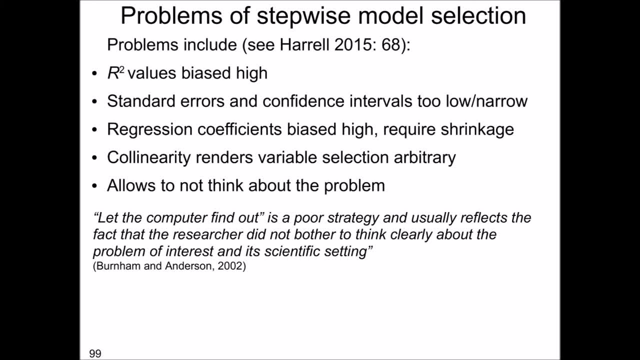 with the full metal And removes variables that are not have no statistically significant contribution to the explained, and this is also captured by this nice quotation from Bernheim and Anderson. They state: let the computer find out is a poor strategy and usually reflects the fact that 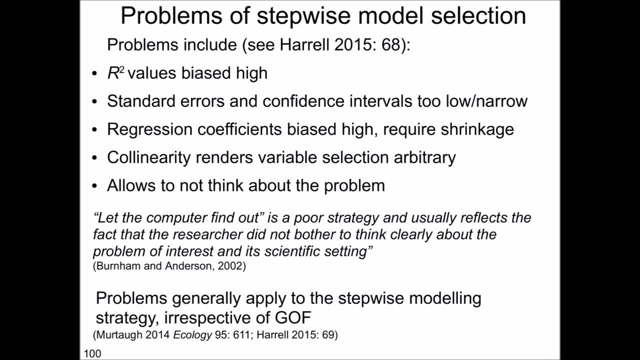 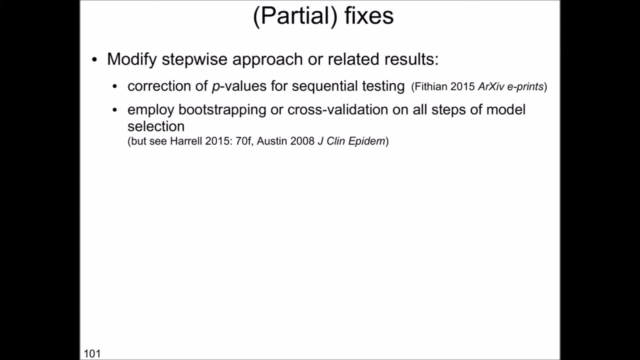 the researcher did not bother to think clearly, clearly about the problem of interest and its scientific setting. We have several partial fixes to deal with the problems that we outlined for the stepwise model selection. One possibility is, if you do hypothesis testing-based stepwise model selection to correct the p-values. 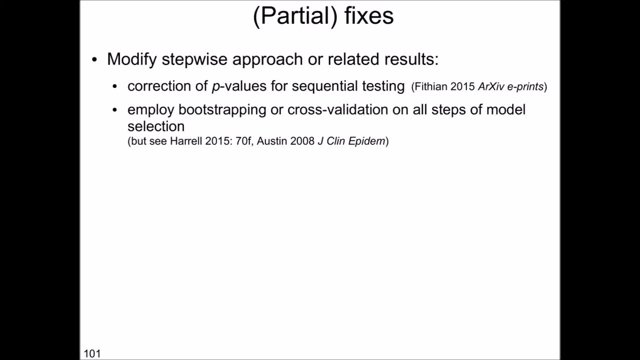 We have discussed that the p-values are biased low and with this correction procedure for sequential testing for the multiple tests that you are doing, you obtain more accurate p-values on which you can base your choice of removing or including variables. Another option is to employ bootstrapping or cross-validation. 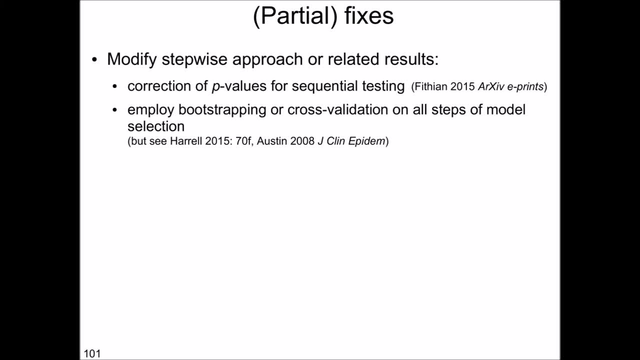 on all steps of the model selection. Bootstrapping means that you draw several samples from your data and you use these samples to run the complete procedure. so the whole stepwise model selection process, and the same holds for cross-validation, where you split your data in the test set and the training set. 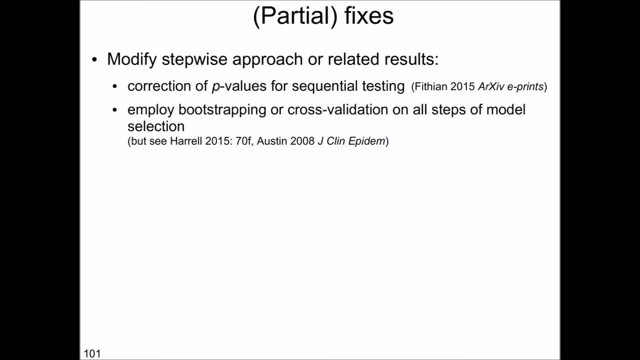 We discussed this before, what cross-validation means, and then you run your model selection process several times and afterwards you can use the results to have a prediction, to predict the observations from your test set. However, as we discussed before, cross-validation is still likely to underestimate the true variance. 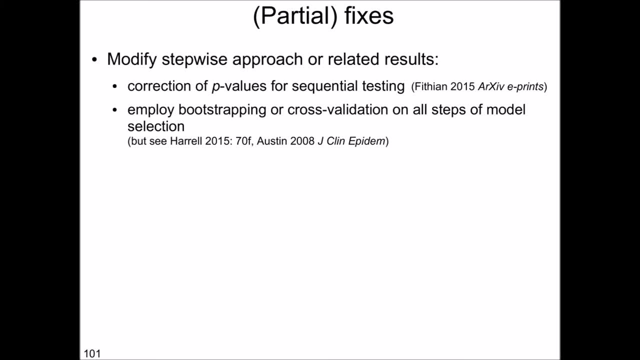 and with the bootstrapping approach, there are several issues. For example, if you obtain different results, which results should you rely on? For example, for different bootstrap samples? you will obtain a frequency: how often the variable is chosen or is selected in the best fit model. 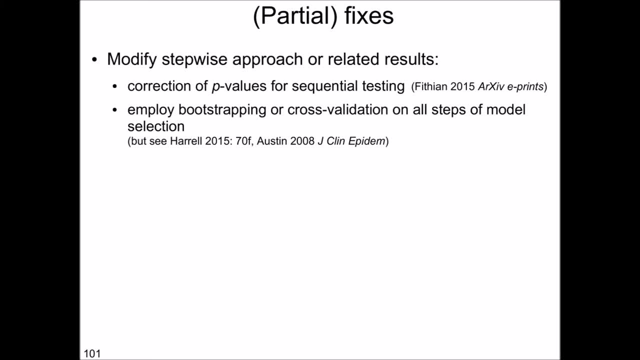 and it is unclear where to set thresholds. In fact, a comparative study by Austin found no improved performance with the backwoods stepwise selection method and in the case of cross-validation you will have to have a switching and backwoods stepwise selection method. 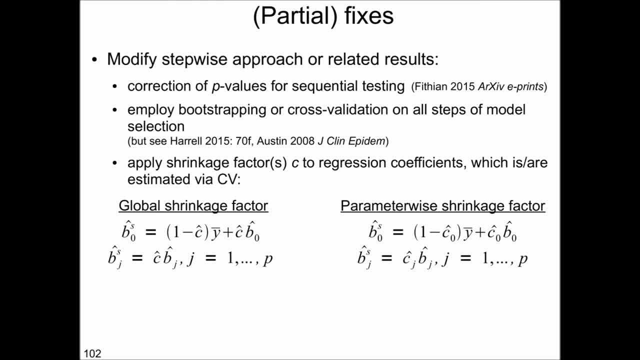 This is why it is so important to stretch the model selection in relation to the backward stepwise selection, to be exactamente consistent. A more interesting approach is to apply shrinkage factors after model selection, and that is called post-selection shrinkage factors, to shrink these regression coefficients. How do we decide on the? 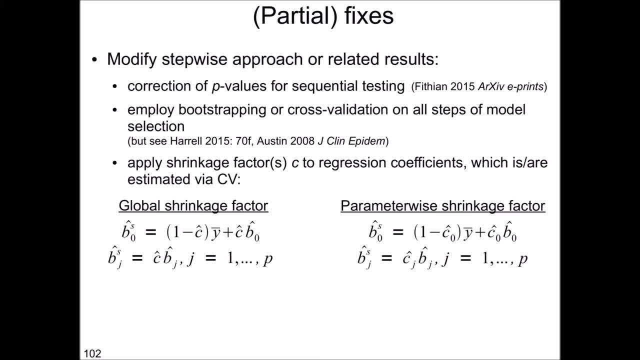 shrinkage of these factors. Well, this is done again via cross-validation. You estimate this shrinkage factors and there are two ways to ask to estimation methods. One is a global shrinkage factor method, where the same shrinkage is applied to all factors and on the other hand, you have parameter. 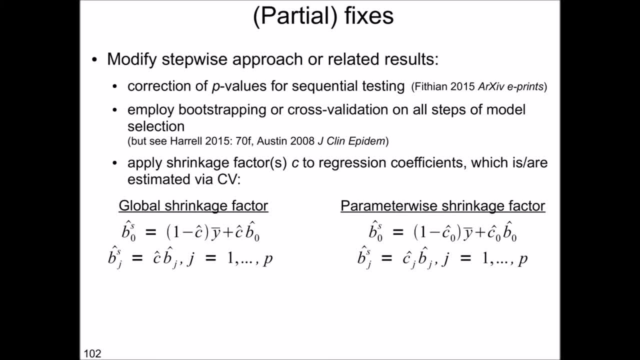 wise shrinkage, where a specific shrinkage factor is determined for each individual regression coefficient. In fact, the recent study found a simulation study that backwards stepwise elimination, so backward stepwise model selection, performed similarly well as another model, Another method that we will encounter soon, the so-called lasso method, when used with 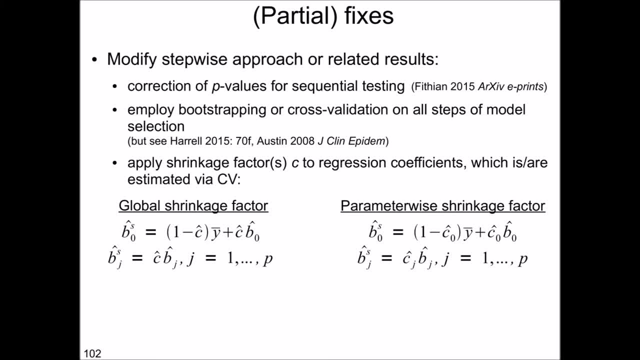 parameter wise shrinkage. So if you want to stay or if you want to conduct backward stepwise, if you want to conduct stepwise model selection, then I recommend to conduct backward stepwise model selection and afterwards to do a parameter wise shrinkage to obtain more reliable regression coefficients. 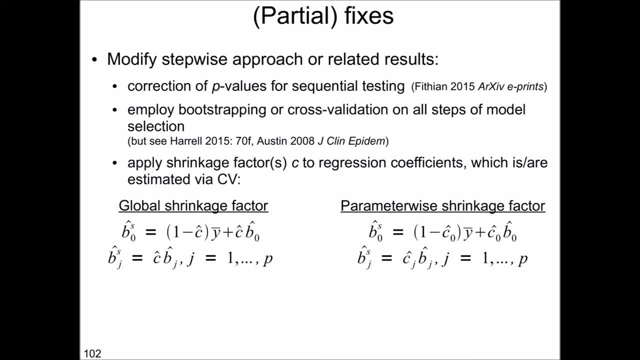 Thank you for watching. And finally, a method that we will discuss further is to use a shrinkage method that shrinks during model selection, So you don't do the modeling and then use a post-selection shrinkage, but the regression coefficients are shrunk during. 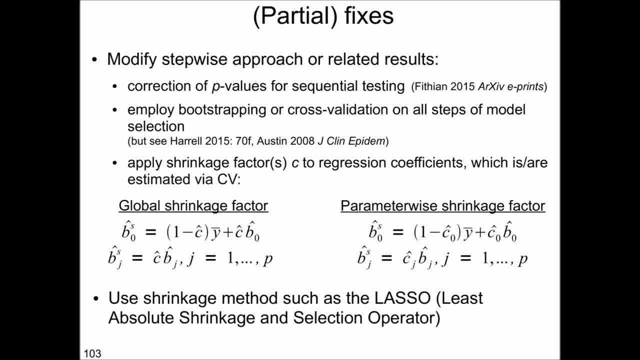 the selection process And the result is a relatively prominent method that has gained quite some attention in the recent decade is the so-called lasso. Lasso is the acronym for least absolute shrinkage and selection operator. So to understand how to use a shrinkage method, you can use the following methods. 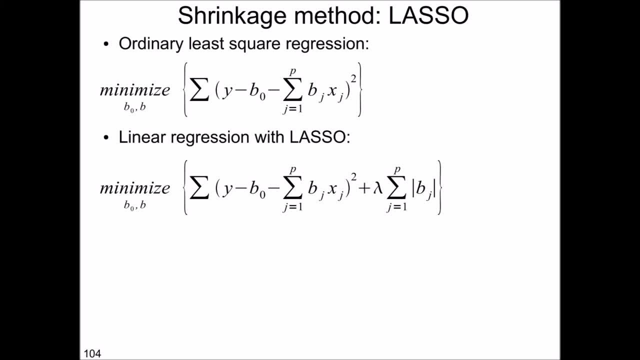 So to understand what the lasso does, we remember what we do in ordinary least square regression. So the linear model, the typical linear modeling that we have already discussed before, what we minimized is the residual sum of squares, And if you would go back a couple of slides you would see that the first line is: 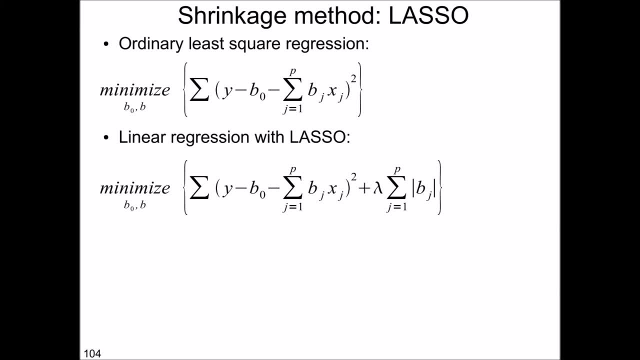 identical to the equation that we have seen on the previous slide, And this is the slide for the ordinary least square regression: optimization or minimization of sum of squares. that has to be done. So we sum up the difference between our responses: the intercept term, beta zero and 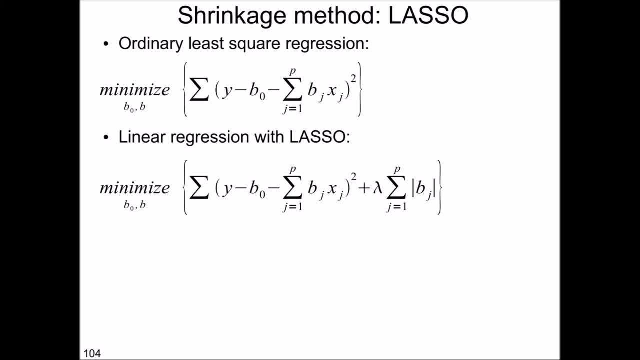 the um, if this is from the original statement that we have our initial case of oliveropobucnrogi- o, g, d, g, q, n, x, q, o, y sum of square errors, or this residual sum of squares. Now let's look what the 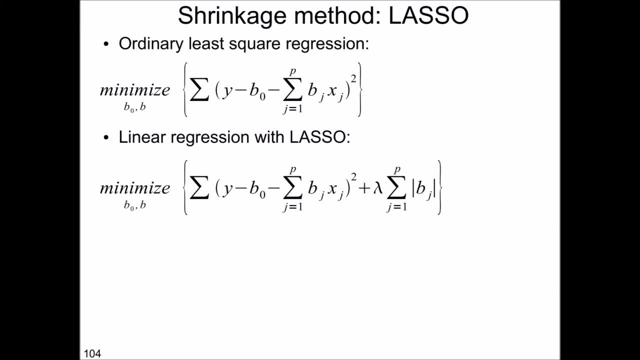 LASSO does The next line linear regression with the LASSO. So the LASSO estimates as well b0 and the beta and the aim is to minimize that. or in fact the b0 is not estimated during the LASSO algorithm, as we will see later on. 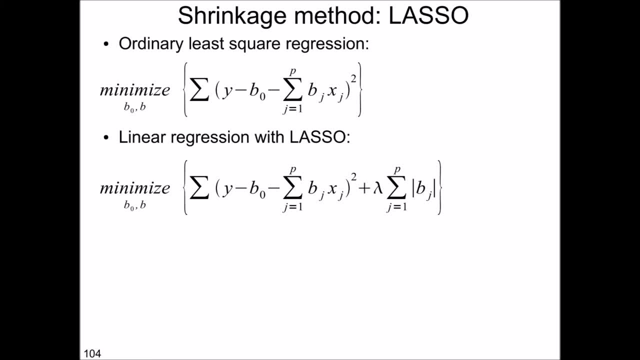 Anyway, if you look at the equation, we see that the equation is the same as for the ordinary e-square regression, but we have an added penalty term, and this penalty term on the right side reads: plus lambda. and then again, the sum from j equals 1 to p for all parameters in the model for all. 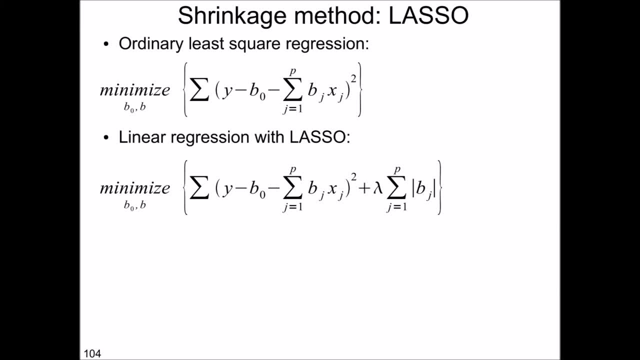 variables we sum up the absolute value of the regression coefficient. I have to say we use a standardized regression coefficient. so that's important because otherwise the scale of the variable would influence this minimization. So standardization here means that we standardize the variable to the same mean of 0 and 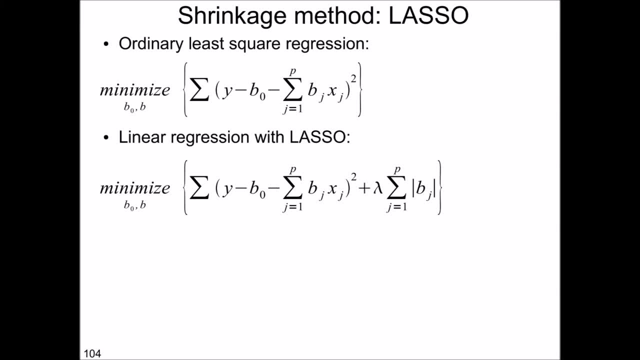 1 standard deviation, And what does this mean? that basically means for the lasso that, depending on the lambda that we choose, we have an incentive. or let's say we don't have an incentive but the algorithm that is run has has an incentive to minimize the regression coefficients towards zero in the end. 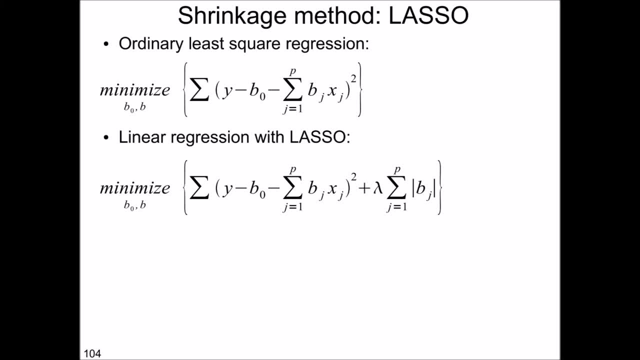 well, why is this done? well, to understand this, we need to know why the method, the lasso, has been implemented. the one motivation of the lasso is that regression coefficients are biased high. we've discussed this already, and this would. this leads to a higher variance in prediction. 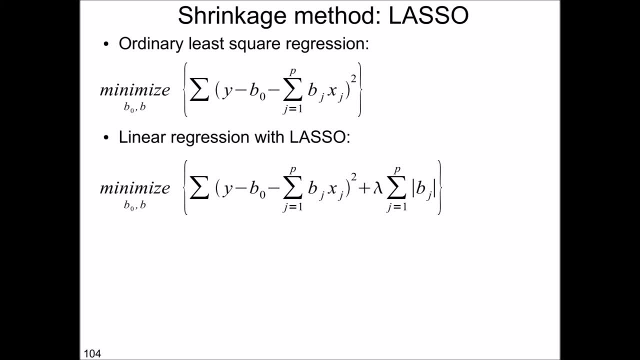 if you have biased high regression coefficients. now, if we, if we shrink the regression coefficients, then this reduces the variance. if we estimate, if we predict a new data set and we have only a slight increase, hopefully with only a slight increase in the bias, and this terminology refers here to what we discussed before with the bias variance trade-off. 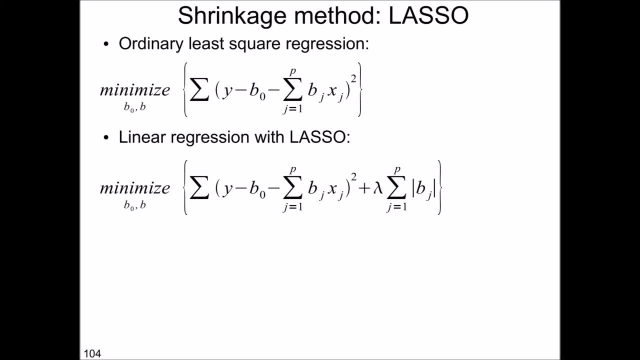 so the first issue that the lasso is motivated for is this: is this regression coefficient shrinkage? and the second one is that for a large number of predictors it's relatively difficult to in to interpret our results. let's say we have 10 or 20 predictors in our model. 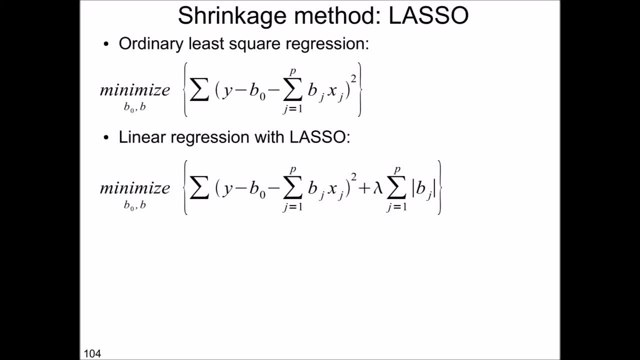 and if we have a regression analysis result where we have 10 or 20 predictors in the model, it's relatively difficult to decide what is. what are the most important predictors and how do i in interpret changes in the response variable? how important an individual predictor, an explanatory? 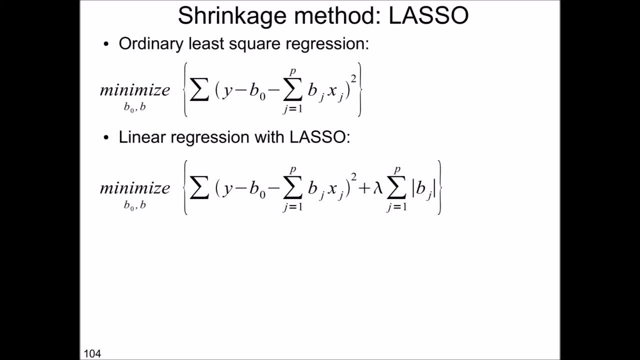 variable is. so you can see that by choosing such a penalty term with the lambda times, the absolute regression coefficients, we shrink these regression coefficients and this solves these two issues. on the one hand, we saw, we have the shrinkage coefficient and on the other hand, we have the 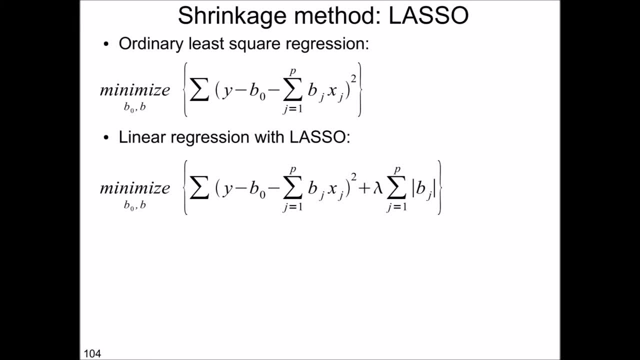 shrinkage of the regression coefficient and, on the other hand, since we can shrink the regression coefficient- and this is the characteristic characteristic, characteristic characteristic of the lasso to zero- we obtain, um, some betas are estimated to be zero and this means we remove a variable from the model. we can. 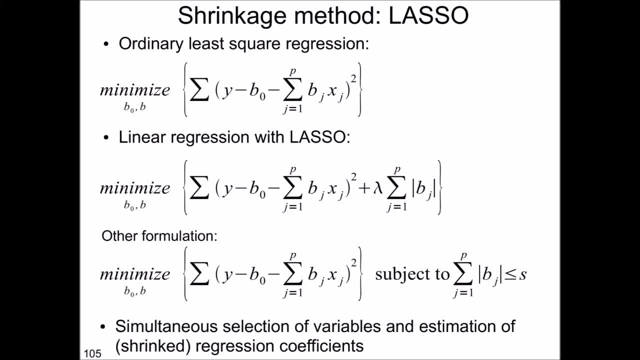 we can also see this when we look at another formulation of the lasso, and this is shown here. so we minimize again the sum of squares of the error, or the residual sum of squares, as they are also called. subject to this condition, to this constraint, that the regression coefficient, the 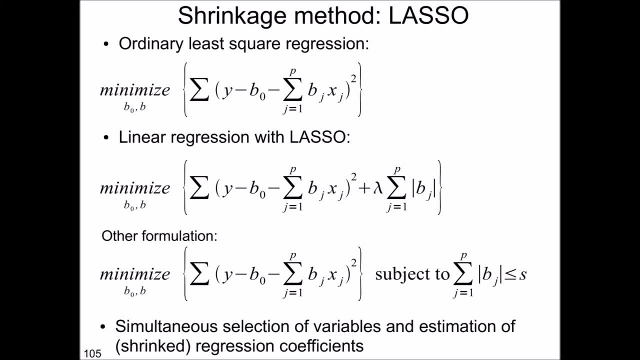 sum of the regression coefficients are smaller than equal than s- and this now is s- to the plus number, which is the total s. the total sum that is allowed means that we have to distribute the soak- you can easily, you can, you could loosely say this budget for the regression. 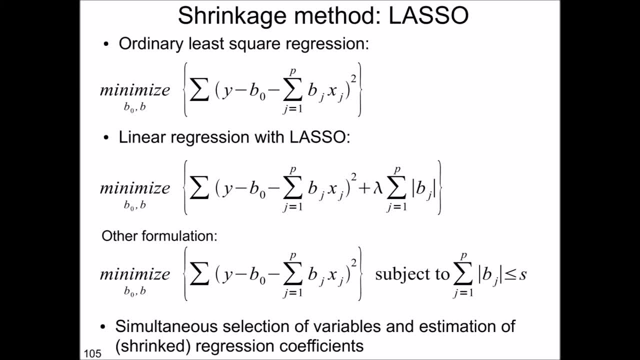 coefficients. we have to distribute this between the individual variables, and this means, of course, that we would give more weight to more important variables than to other ones, and then we that we be able to shrink some of this betas to zero. So what this all means is that LASSO does at 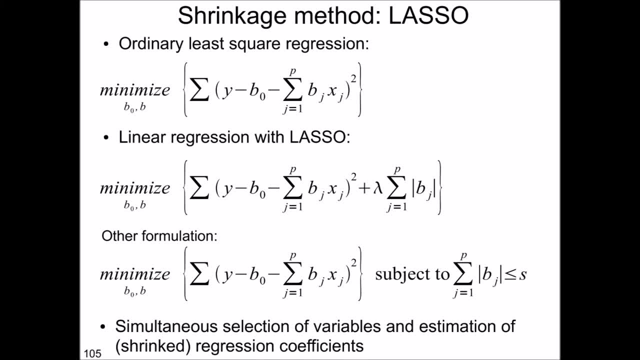 the same time, a selection of variables and estimates shrink regression coefficients And, in fact, while this looks not very exciting to you perhaps, in the and on first encounter, this technique has been found to be really high performing. It has among the lowest prediction error when compared to several other techniques, and I recommend that you do a little bit of more. 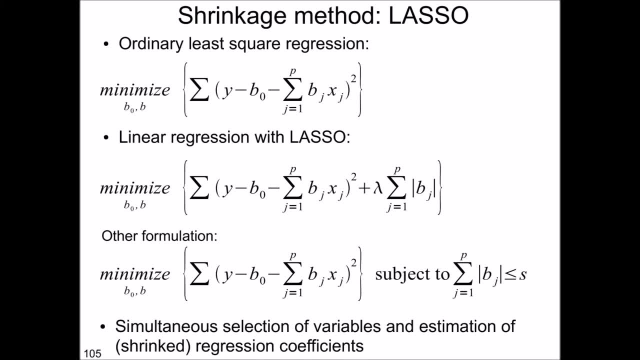 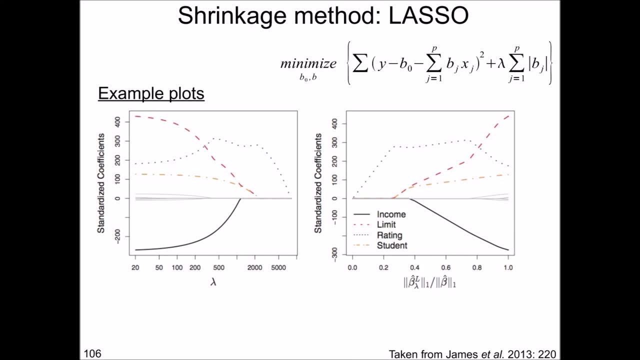 of the reading of the literature sources that I provide to you in the notes to this slide. So let's quickly look how this looks like. Let's take a quick look at the result from a LASSO procedure. So when the LASSO has been run on a regression problem, and we have here, I'll just 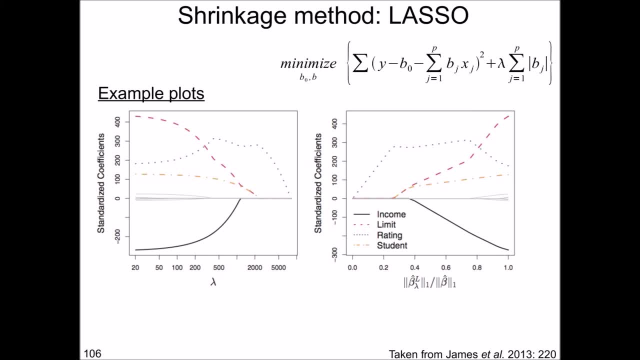 show you for easier understanding the equation again on the top right of the slide. And we see that in this equation, as mentioned before, we have a lambda that is set on the x-axis and a lambda that is set on the y-axis. and when we look at the 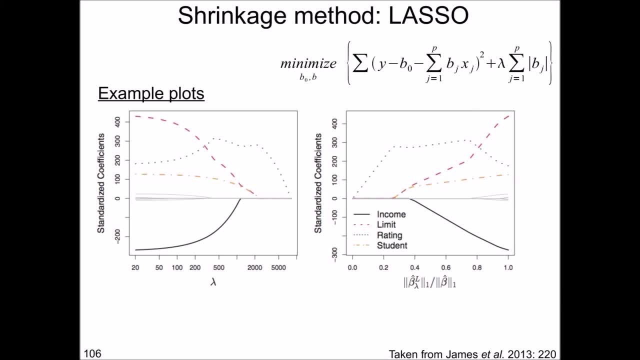 left figure. we have lambda on the x-axis and we have the standardised regression coefficients on the y-axis. So we have the change in the regression coefficients plotted against lambdas for four variables. Several other variables have been included in the model before, but they are shrunk to zero and are not explicitly shown here. They. 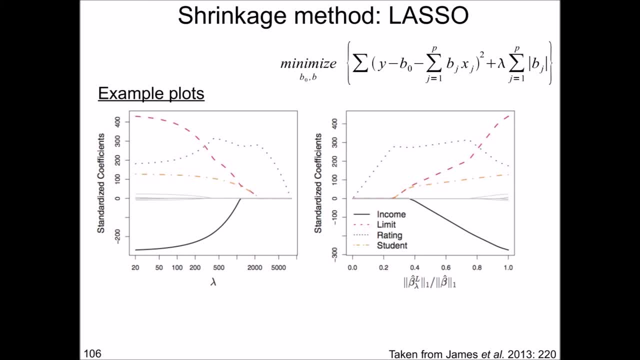 are all gray around the x-axis, They are just grayed out. Well, what you see is that these four variables, the regression coefficients of these four variables, except for the blue line, for the blue dots, decrease to zero when lambda increases, Eventually, when lambda becomes very large. 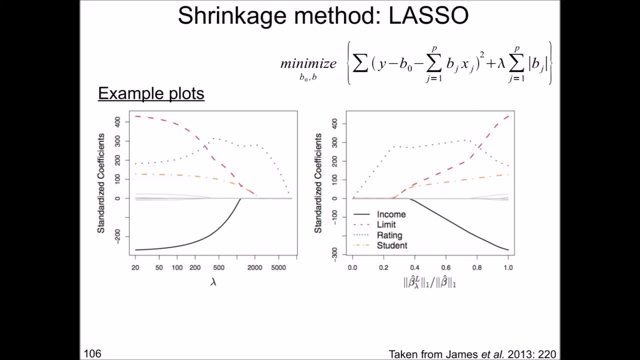 for example- in this case it's a logarithmic display on the axis probably around 10,000 or something- all variables become zero. All regression coefficients of the variables become zero. This shows that depending on our choice of the lambda we also have, for example, if we choose a lambda of 5000, we would 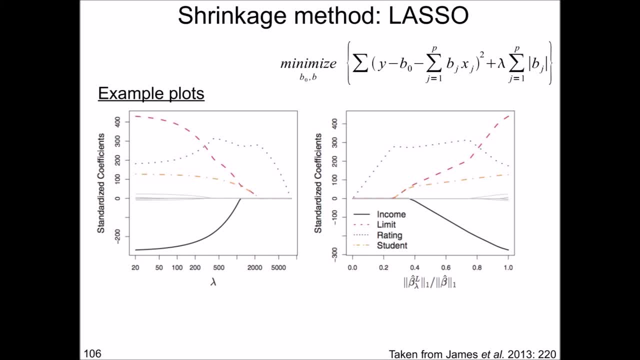 only have one variable. in the model On the right side we have a different graphical display and this is the same regression coefficients for the same variables shown against the total sum of the regression coefficients, The total makan. absolute sum of the regression coefficients for the ordinary least squares equation. 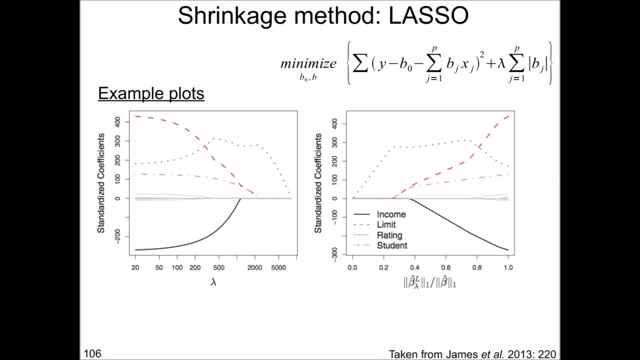 So in the beginning, when we have almost no penalty. so the lambda is very low, of course. the absolute, the total absolute sum of regression coefficients from the ordinary least square regression and from the lasso regression are the same. they are run. So we move here with 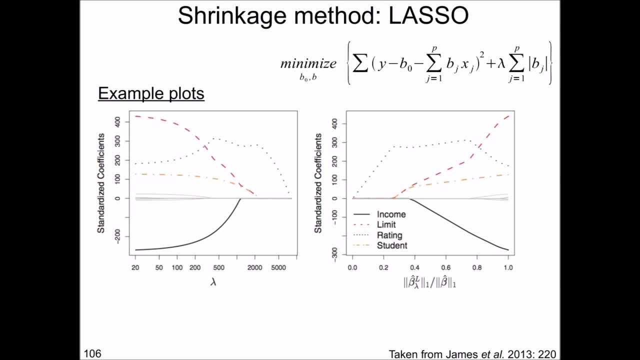 an increasing lambda from right to left. so one means that the total sum is the same and if we increase the penalty term, we see the same movement or we see the same change in the regression coefficients as on the left. plot from only here, from right to left, and we approach zero for all. 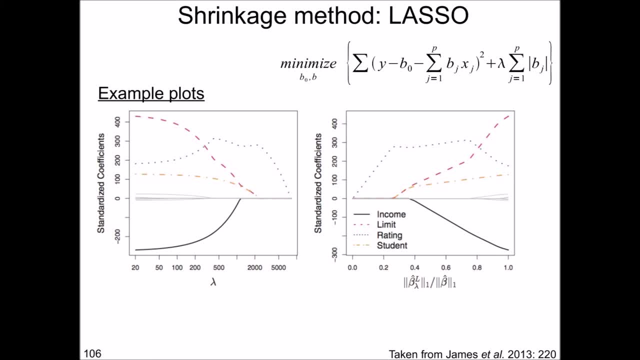 these regression coefficients at some stage. So we have to ask ourselves: okay, this is all very nice, but how do we identify the optimal lambda? because every, as we see here, the traces of the different lambda show us that there's several options for choosing a lambda, depending on which lambda we 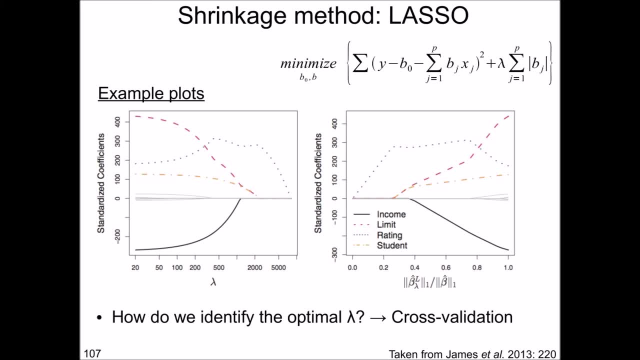 choose. We have one or three or more variables in the model, so which lambda should we choose? and this is done via cross-validation. So how does this work? So, after choosing several lambdas, the algorithm runs and returns the results as shown here in these plots, and then for these results, we can estimate for each of. 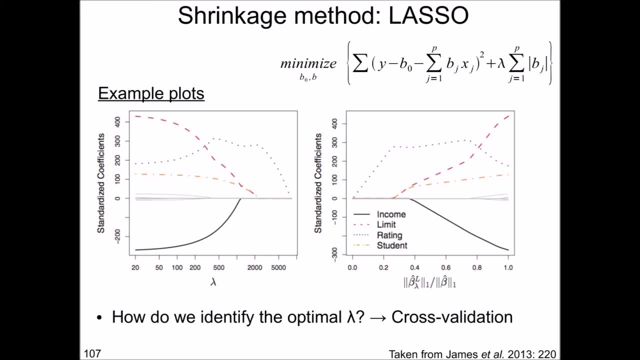 them, at least for several points of these results. we can estimate the prediction error using cross-validation, and we do this in our in the demonstration. and an optimal lambda minimizes the prediction error. So we choose the lambda that minimizes the prediction error, and then we have 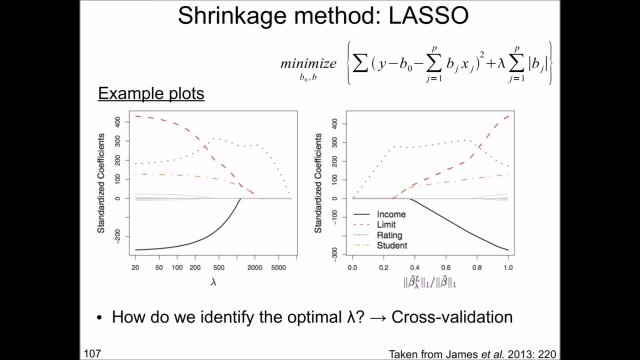 one definite lambda, For which we can then take the regression coefficients and have a solution for our procedure. So overall, as I mentioned before, the lasso analysis is really a method that performs really well and should be used when you have many variables and you have 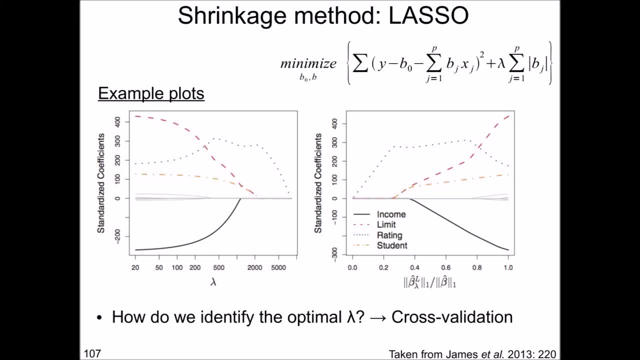 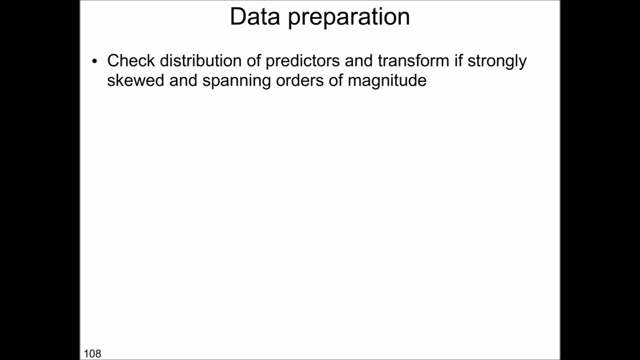 to, or you want to, explain why which variables are important for an observed phenomenon. So now we approach the end of our session. today we have discussed several topics, starting with modeling strategies, and we end perhaps a little bit strange, But I think it's more important to first understand what we are doing, and we end with a little. 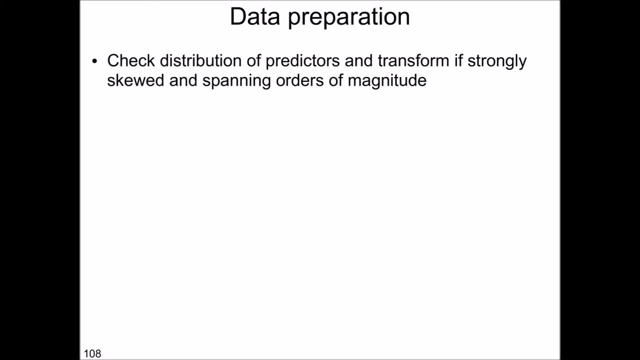 discussion of what we actually need to do before we start the modeling, And one of the first steps is data preparation. and this may be known to you already from previous sessions in statistics that before you start modeling you have to inspect your predictors, your explanatory variables and, in case 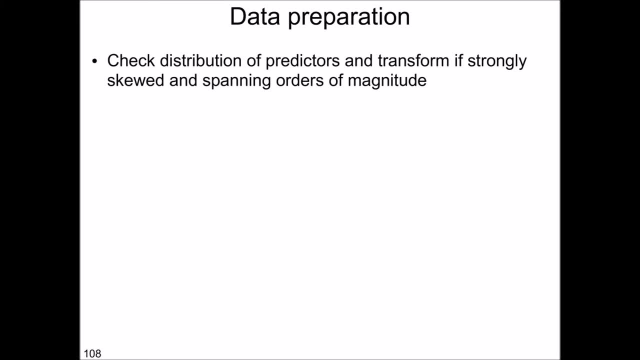 that you have predictors in the model that are strongly skewed or and span several orders of magnitude at the same time, then you should think about, or you should decide, whether you would want to transform these variables, for example, log transformation or a square root transformation, depending on the data. Now, one type of data that often exhibits skewed distributions: 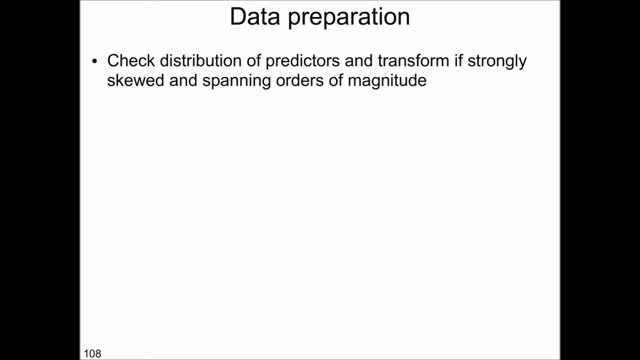 are chemical data, Where concentrations may easily span orders of magnitude and often relationships with ecological systems are existing on a log scale. A more important issue that you have not encountered before is so-called multi-culinarity. Multi-culinarity means that there's a strong correlation between explanatory variables, and if you have such a 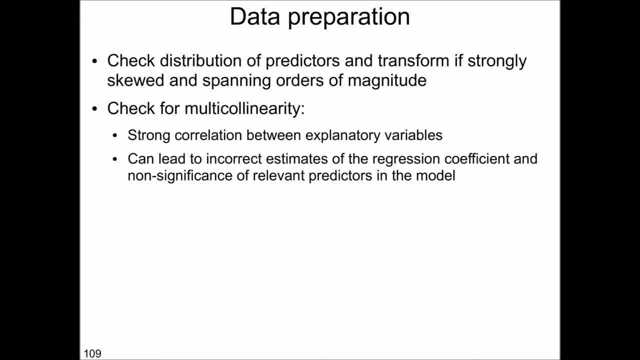 correlation between explanatory variables, then this can lead to incorrect estimates of the regression coefficients and non-significance of relevant predictors in the model. For example, in stepwise model selection, only one of the important predictors is chosen. this can then be happened randomly and you don't know whether this variable is really important. 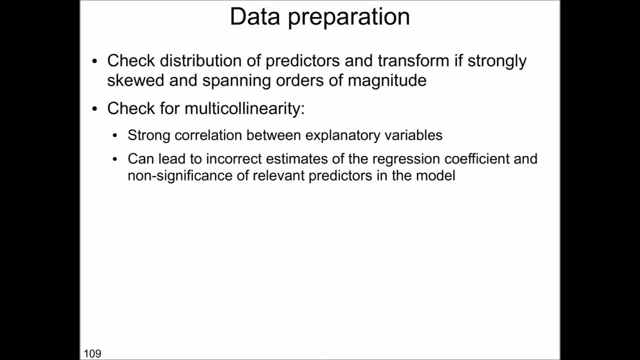 or whether another variable that has not been selected but is correlated would in reality drive a specific process causally. Generally, multiculinarity does not affect predictions, so if you have a data set and you include, for example, both culinary variables, you then have direct correlation with the data. The result of this is therefore a random increase in a particular variable. However, if you don't have a prediction method and you need to calculate all the calculations that you want to do in your model, you can also use this kind of method. For example, on the other hand, you have a data set that you use, for example, both culinary variables. 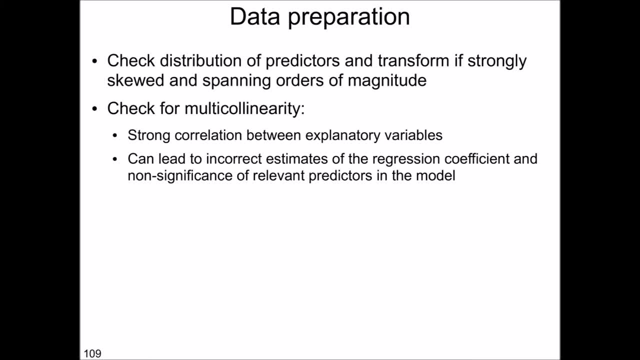 So you can also use a formula that your data set is not about the three variables but, in this example, the, a data set where you include, for example, a particular number of variables and then use the same variable variables, then this does not matter for prediction, at least as long as the variables exhibit. 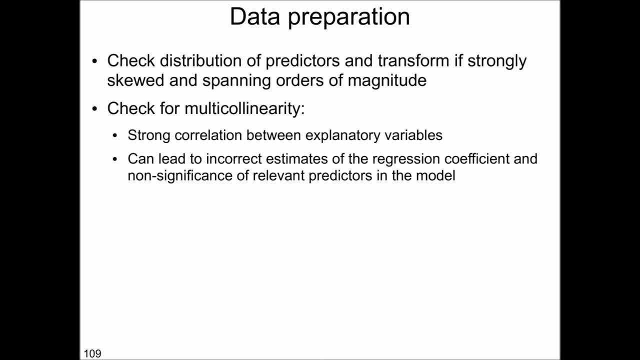 a similar culinarity as for the original data. So, for example, some variables that are often correlated are nutrients and conductivity and aquatic ecosystems, And when you have this correlation between these variables, you can be relatively sure that this correlation also exists in other data sets. and if your aim is to predict a 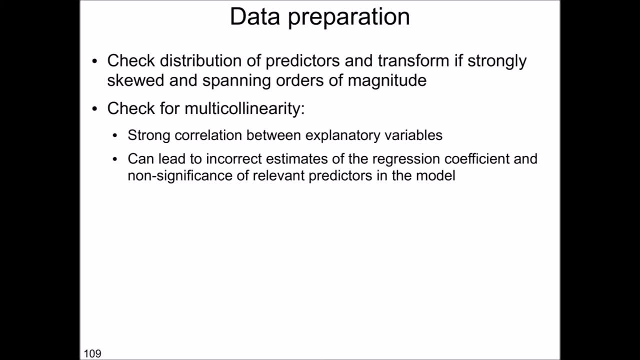 phenomenon specific response, then you can keep both of these variables in the model. If your aim is explanation, you run into a problem here, because if only one of the variables is chosen, you don't know which one is really important. And if it's then a correlation between these variables, then you can be relatively sure. 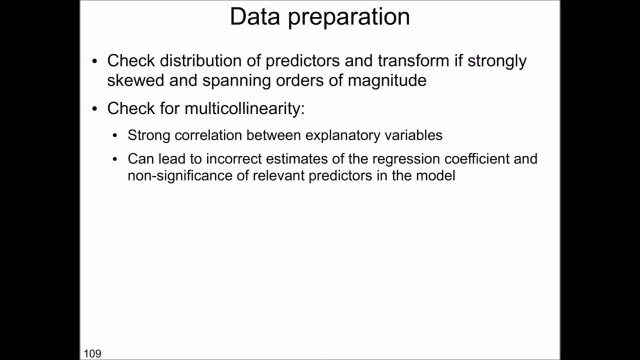 that this correlation also exists in other data sets and if your aim is to predict a phenomenon, specific response, then you can keep both of these variables in the model. If there is really high correlation, then you really can't decide based on the statistics which variable is important scientifically. 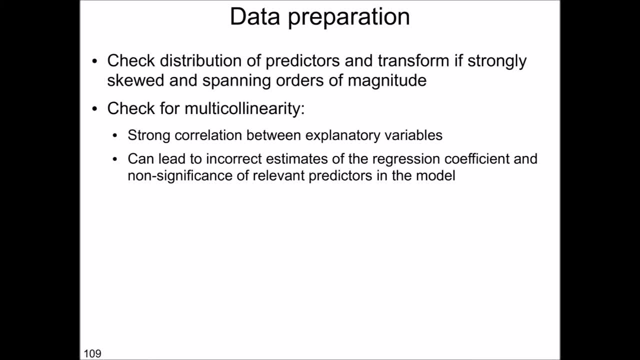 That is not possible. How can you diagnose culinarity? Well, this is done through visual inspection. You can. You can plot the variables and look at the scatter, at the relationship between on the b-variant case. Same can be done if you do a correlation analysis or calculate correlation coefficients. 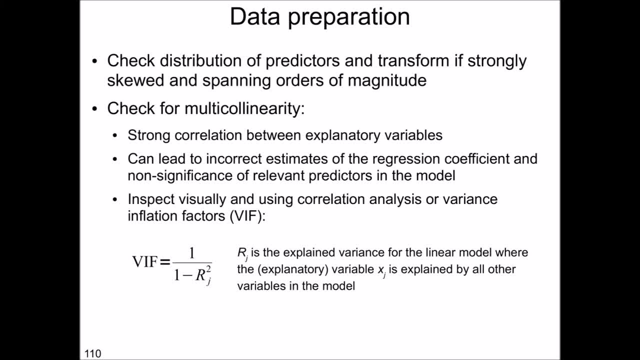 or of course you could also- and this is most recommended- you can do a variance calculation of a variance inflation factor, so-called VIV, And the calculation of the VIV is shown here. the equation: the VIV equals one divided by one minus r-square. 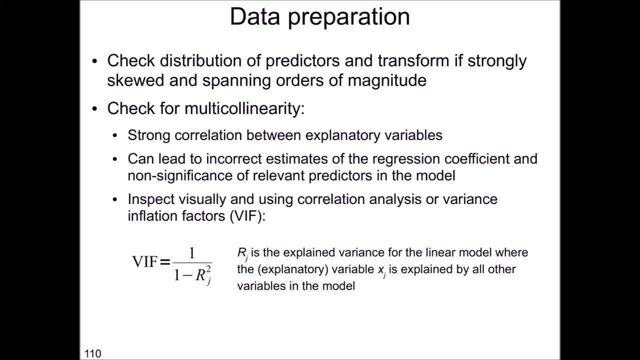 And the r-square refers here to the explained variance for the linear model, where one explanatory variable is explained by all other variables in the data set or in the specific model. So let's say we have a data set with ten variables- explanatory variables- that we want to use. 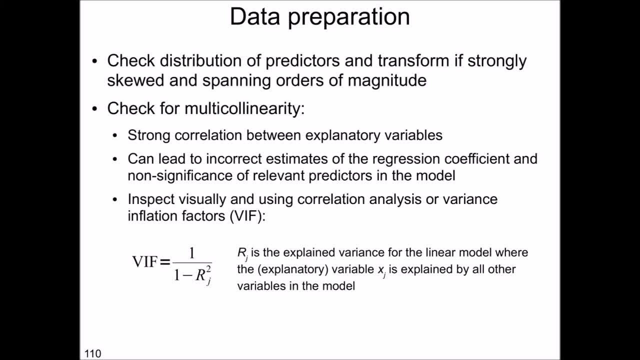 to predict. as response, then, for the calculation of the variance inflation factor, we only focus on the ten explanatory variables and we take each of them and try and calculate this with if they, if this variable is predicted by all other explanatory variables and the rest of them. 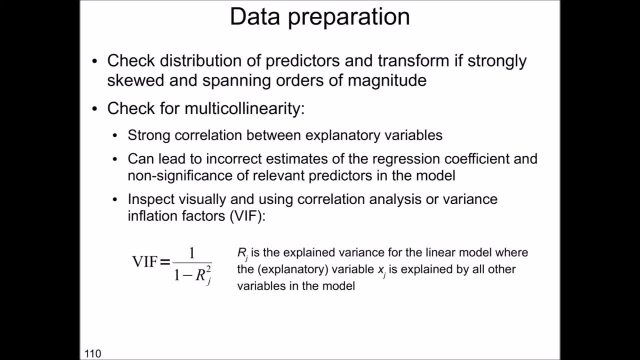 The rational is quite clear. if we have a very high r-square, so all other explanatory variables have a high proportion of information that can be used, that that is sufficient to explain the remaining explanatory variable that could, then we could as well remove it from the model, because we don't lose much information and we can see, for example, 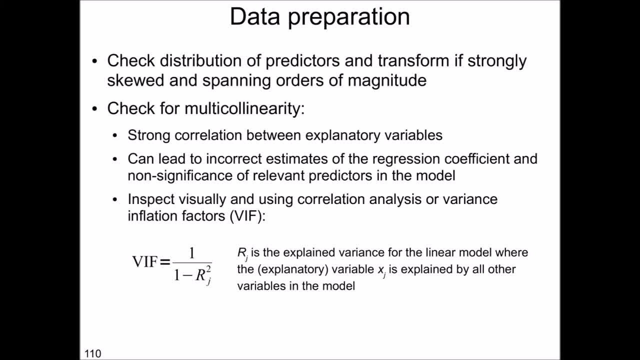 With The, this r-square. if with the r-square approaches one way, the denominator becomes smaller and smaller and then the variance inflation factor increases. and this is also what the what, what the textbook say: if you have a variance inflation factor above four Or Above, 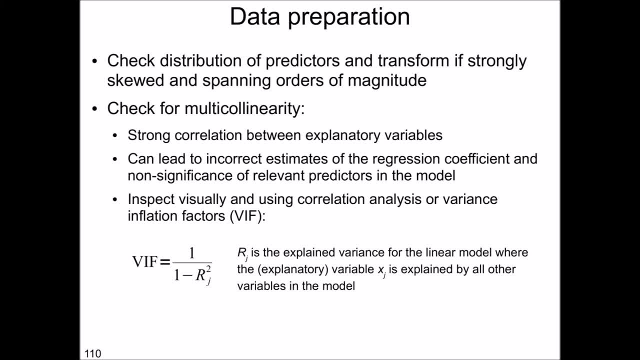 Five, Some other say above ten, then you really have a problem of colinarity you should be worried about. Why is this the case, of course? well, how do we obtain a variance inflation factor of five? well, five is obtained by dividing one By zero point two, and that basically means that you have 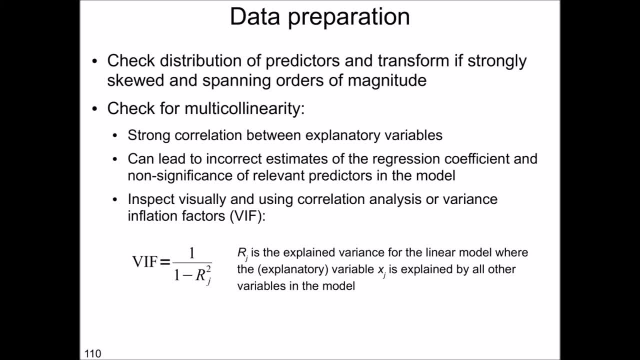 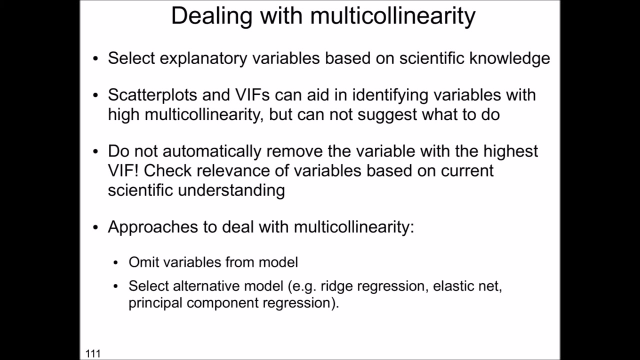 One minus zero point eight. eighty percent of the variance in one variable is explained by all other variables, so there's not much unique information in this specific variable. So how should we deal with the multicolinearity? well, first of all, always when you do a statistical 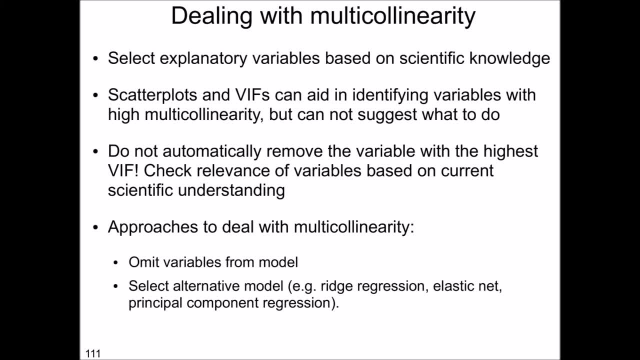 modeling. Do not just include all the variables that are available, but select your explanatory variables based on scientific knowledge. screen the literature and check which variables are known to be important to explain a certain phenomenon. Secondly, scatter plots and whiffs can aid in identifying variables with high multicolinearity. 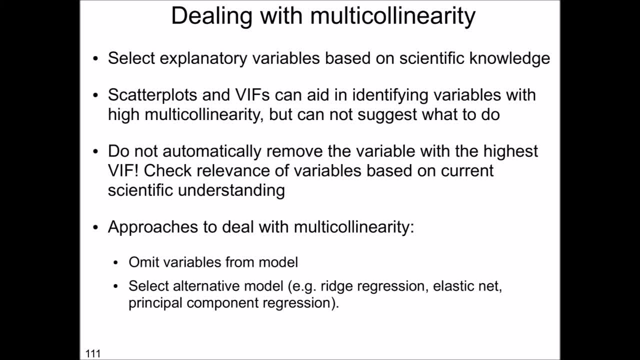 but they cannot suggest what to do. So. So this means You have to think about the result And you should not automatically remove the variable with the highest variance inflation factor. It can be that, for example, one variable has a high variance inflation factor but is very 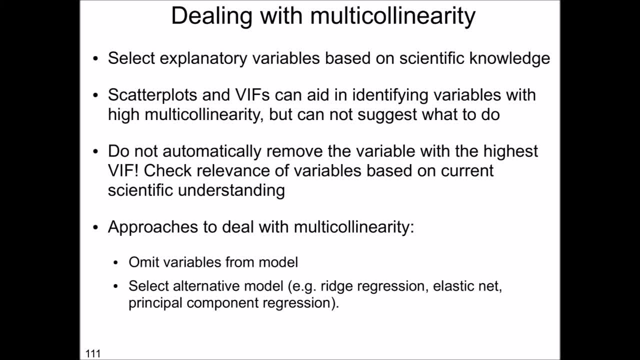 important for the response that we are studying and you, rather, would remove two or three other variables that are less important for the Response Variable, for explaining the response variable, but are confounded, so have a high correlation with this variable that has been indicated with the highest width. so we need to understand. 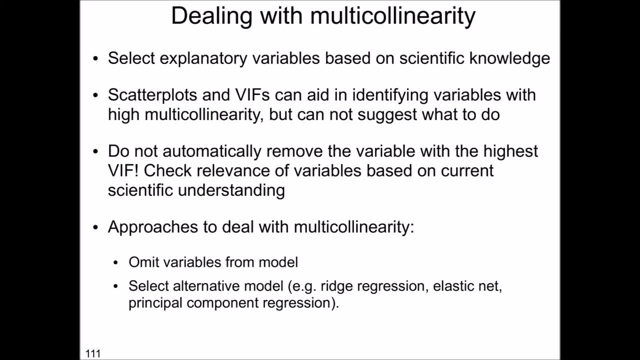 scientifically what we are dealing with, to really make sense of the results from multicolinearity analysis. So So, So we deal then with multicolinearity. One potential option is to omit variables from the models. check which variables have a high heurens inflation factor. you look what is the correlation structure with other variables. 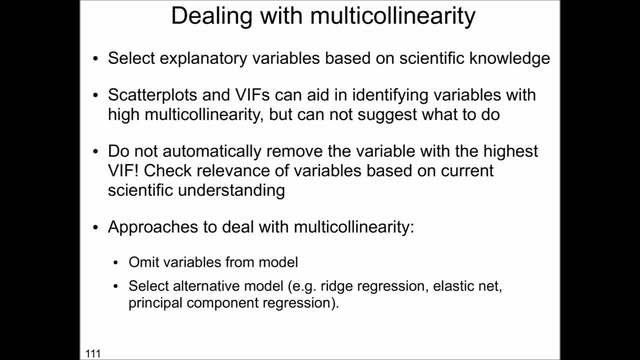 and then you see Which ones of these variables you omit from the model based On expert knowledge. There are also other models that can be used, so, instead of relying with a regression model, with the ordinary e-squares regression model or another one where you know that you have, you run into this problem, and this is. 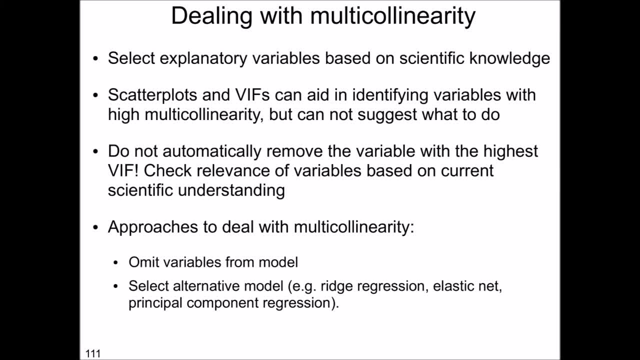 for example, also the LASSO- would run to a problem. here You can select alternative models, and one model I just want to mention here is a ridge regression. that's actually relatively similar to the LASSO. The difference is that you choose a different penalty term and the so-called elastic net that we 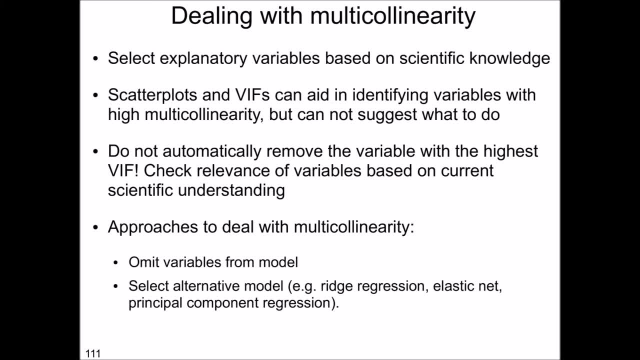 will briefly discuss later again, is also a model that has is quite familiar with or related to the LASSO and ridge regression, because it combines the two penalty terms of the LASSO and the ridge regression. So in case that you have a very culinary data set, you should not use the LASSO, but you should rather use ridge. 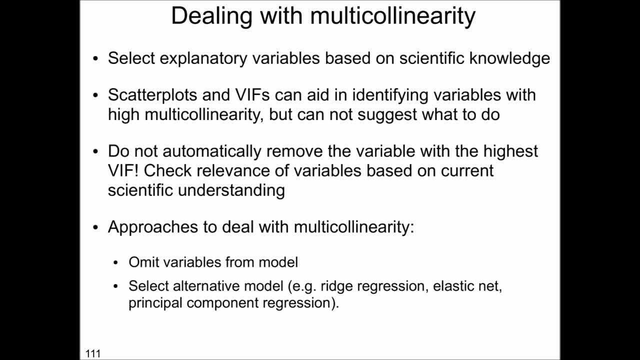 regression or the elastic net for the modeling process. Principal component regression is another option that you can use and principal component regression is a principal component. analysis is first conducted Where you identify new variables that are orthogonal to each other. so they are, they have no correlation with each other- and you extract these. 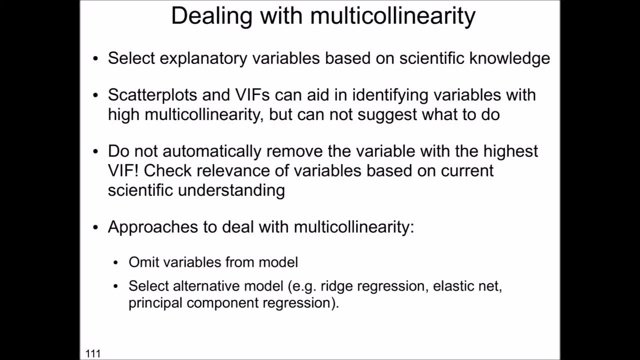 variables from your original data set and principal component analysis is later discussed in this course in more detail. You find different comparisons. you find comparisons of these different methods in the notes to the slide. some links to that. Interestingly, analysis of Dorman et al on culinarity found that while we have this very 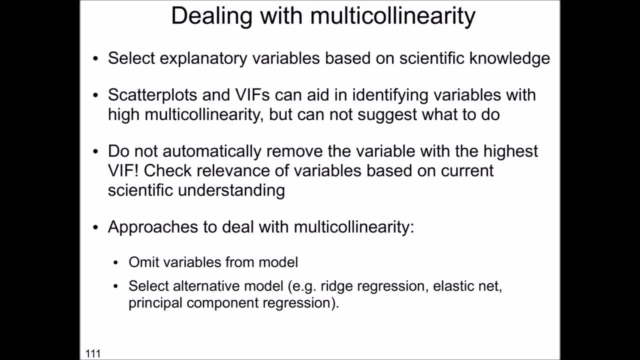 sophisticated methods like ridge regression that just using a threshold based on regression coefficients to decide on that based on expert knowledge to omit one of the variables from the model, works Similarly well. so you don't necessarily need to use these very sophisticated methods if you have a good understanding of the system. 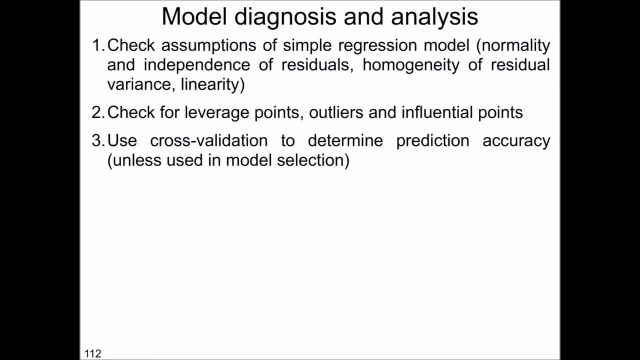 Now, when we have gone through all steps of modeling, we obtain, in the end, final model, and this model still needs to go through model diagnostics and the first thing that you, for the first thing that you always do is to do the analysis that you always do is to check the assumptions of the model. luckily, in the case of multiple, 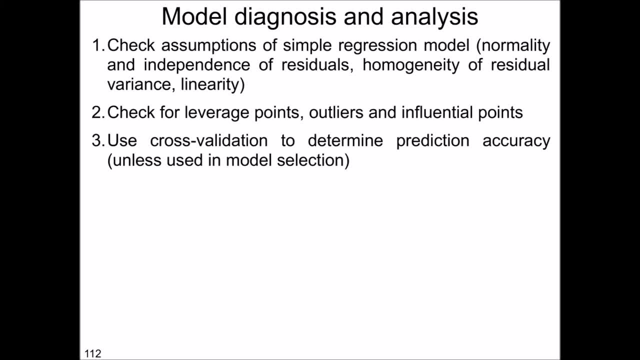 linear regression the assumptions are the same as we have already encountered for the simple linear regression model. so first of all you need to check the normality and independence of residuals and, as we mentioned before, that's particularly a problem if you have temporal or spatial autocorrelation, so if you sample unit the same units in the environment again, 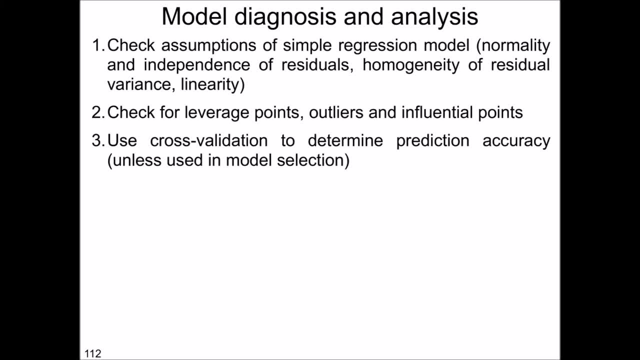 in time or in space, and if this is the case, you probably need to use more appropriate models, such as the generalized least squares model. other issues maybe that should be checked are homogeneity of residual variance, linearity, and in case you encounter non-linearity or non-normality- and we will look in r how to check this- then 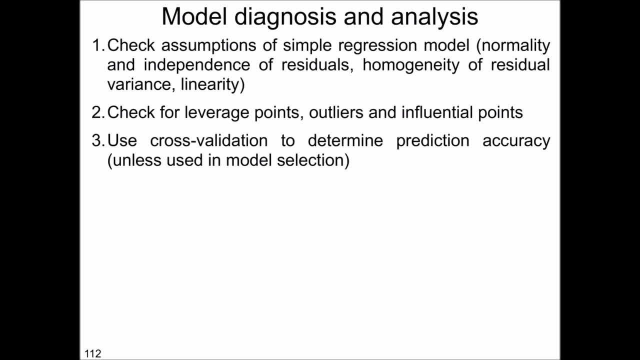 you may want to think whether the model that you've chosen is really appropriate for your data- data at hand, for example for count data or for abundance data, generalized linear models are often more appropriate and if you have such data and can model this data more appropriately with, 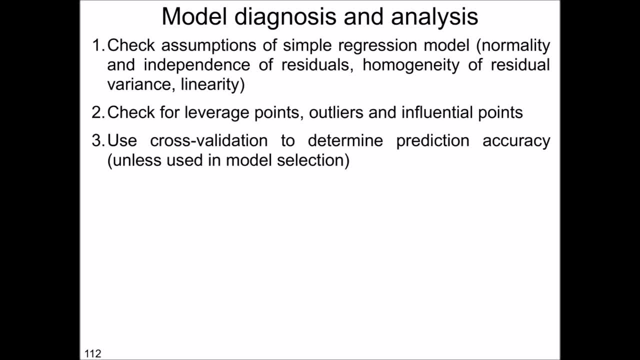 a glm, so generalized linear model, and this should be done, should be done. so we discuss more in more detail the glm in the next session. in the literature it has been suggested that this is a type of data that is actually not dependent on a particular variable, and it 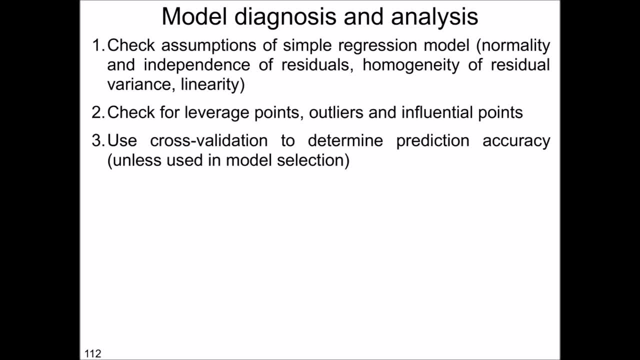 has been suggested as well to transform the response variable, but you should only do this if you cannot find a more appropriate model that can deal with that type of data. another issue that we've also discussed before is that you need to check for leverage points, outlines and influential points. all of this has been discussed in previous parts of the 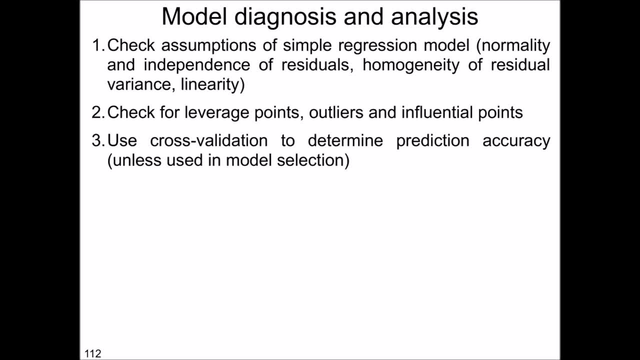 you already used it in model selection and of course you don't need to use it again. Otherwise, you have to determine the prediction accuracy with cross-validation to obtain more accurate estimate of your prediction accuracy for a cross-validation, So optimally 5- or 10-fold cross-validation should be used. 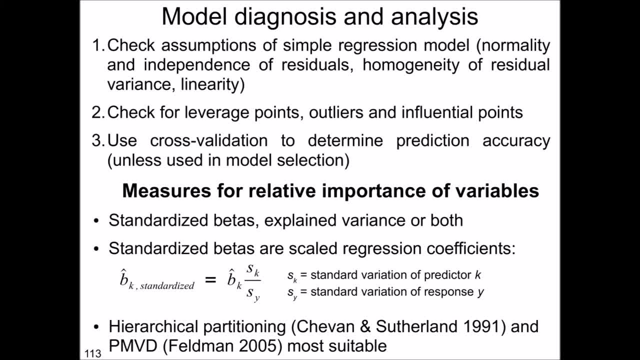 Now that you have your final model. unless you have a model that already informs you on the importance of individual variables, for example, as in the case of the lasso, then you may want to determine the relative importance of variables, for example in simple. 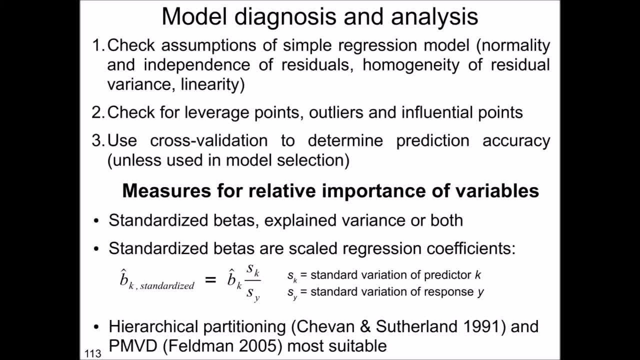 linear regression models, and there are different measures have been developed to do this. They are either based on standardized betas, so on the regression coefficients themselves, or based on the explained variance, or on both metrics. So there are also measures that combine both of these. 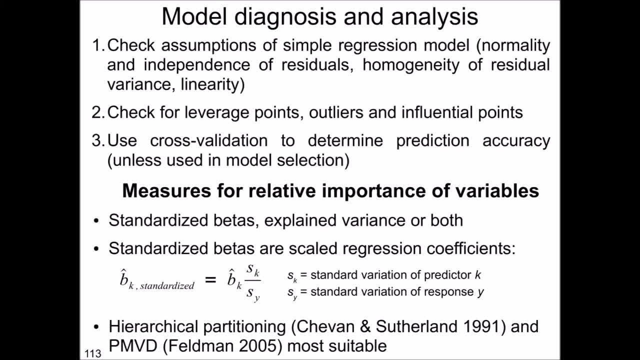 Standardized betas are generally contested because they are not related to partitioning of R-square and they only measure the individual contribution to the model based on the regression coefficient but not directly the explanatory power of a model, which may be especially problematic if you have collinearity in a model. 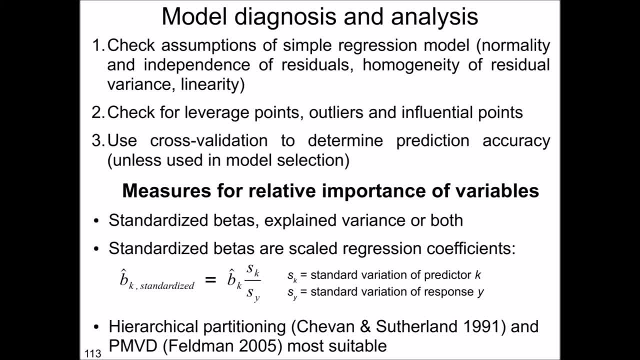 you have discussed before. So standardizing betas is relatively straightforward. It's shown here. So you obtain standardized betas as scaled regression coefficients by multiplying the regression coefficients with the standard variation of the predictor divided by the standard deviation of the response. What is nice for these standardized betas? 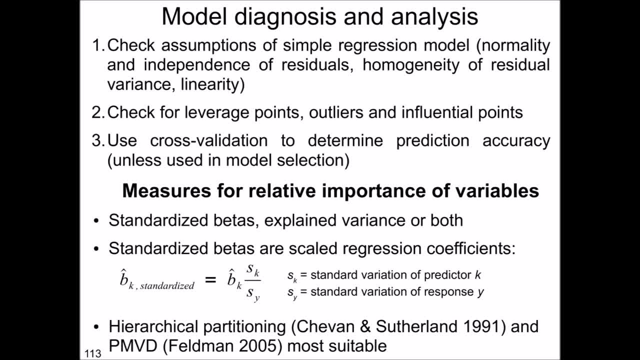 is that they inform on the change of the response variable for one unit change in the predictor. However, as just discussed, they are not ideal and I would recommend to rather use hierarchical partitioning. or there are different methods. It's PMVD. We don't go into details here in the 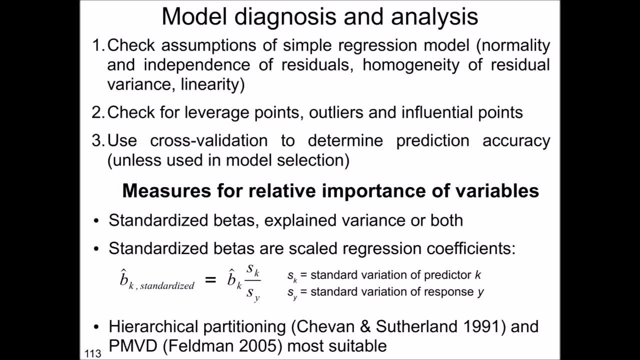 latter method. You can look into the literature Or into the R package to calculate this one. The hierarchical partitioning basically determines, for each variable, the joint and unique variance that is explained by a particular variable and should be used if you use the stepwise modeling procedure based on ordinary least squares. 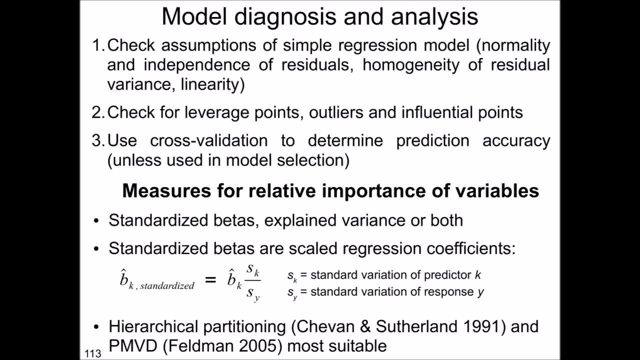 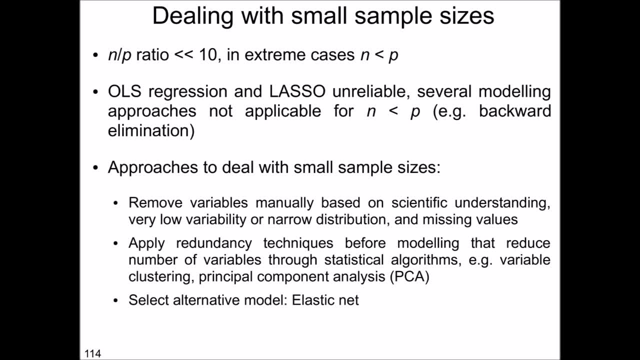 regression. The final issue that we want to discuss is how to deal with small sample sizes. So most of the methods that we have discussed before are mainly tailored for the situation that we have at least 10 observations per parameter in a model. The more 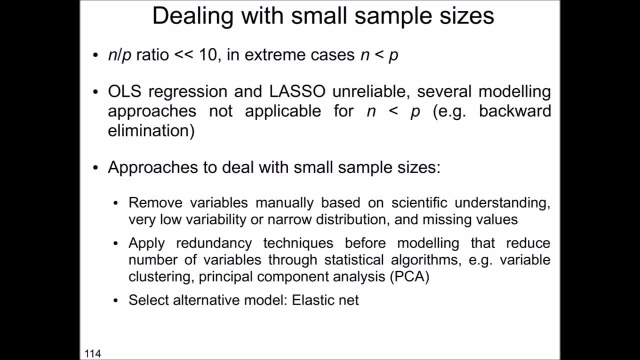 the better, of course. But what do we do if we have much less than 10 per parameter? So let's say just five, or we can have extreme cases. So let's say just five, or we can have extreme cases Where we have less observations than parameters. What do we do then In these situations? 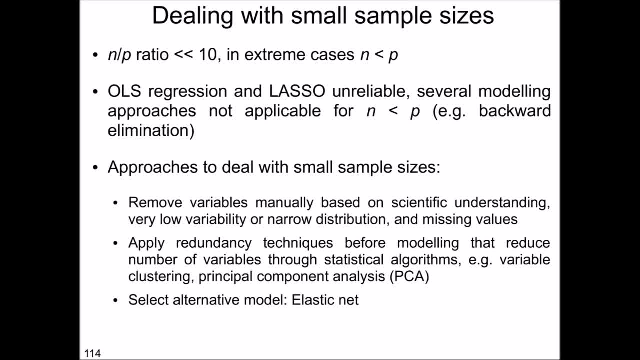 ordinary least squares. regression is really not applicable. We cannot fit a full model in this case. We cannot run stepwise backward selection. We cannot run the lasso. It does not result in ideal solutions, So we need different techniques. One option to deal with that is to remove variables. 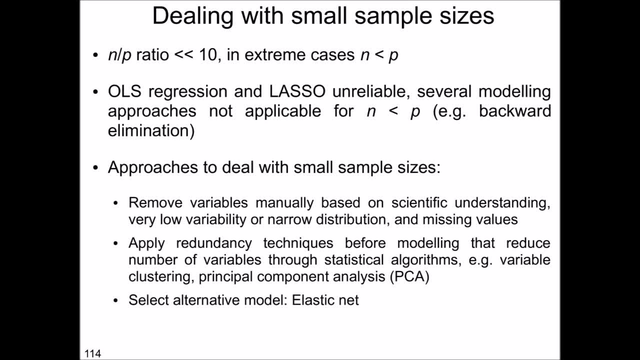 manually, based on scientific understanding. So if you have too much parameters in the model, of course you can just get rid of some parameters, and this can be done, of course, always based on scientific understanding. Maybe there are several different kinds of R. Can we run that? Can we do? 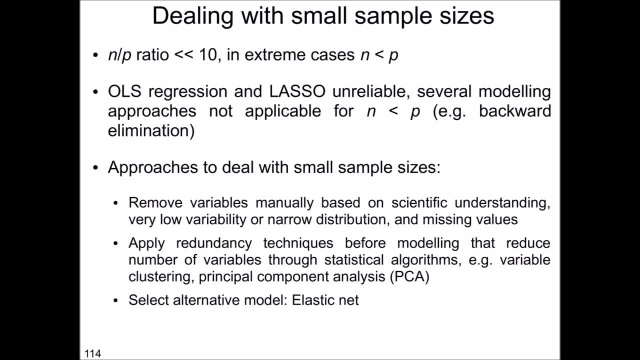 it? Yes, we can. Let's see variables in the data set that are not really needed, or you have very low variability or a narrow distribution for some data. for example, if you have chemical measurements, we may have many chemicals in the model that have many data where they have not been found, so we have 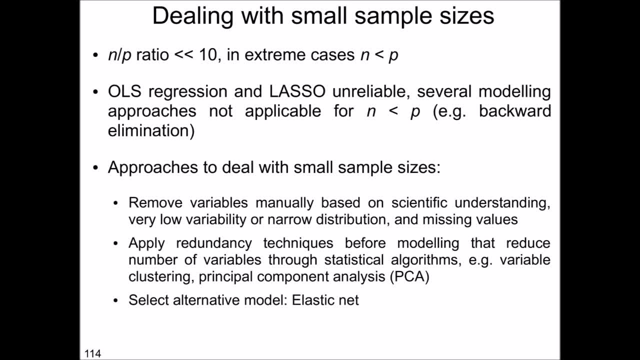 just non-detect- that are assigned, sometimes assigned certain values, or we are sure that they have more or less, are not occurring in the system and we have just two times chemical concentrations in, let's say, 50 or 60 for 60 or 60 observations. we have such a variable. 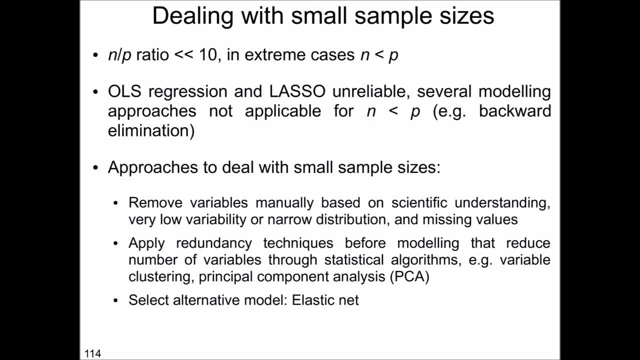 that has always non-detect and then two times finding, then we can be relatively sure that it will not explain much of the variance in the response variable, unless the response variable is more or less a constant. The same holds, for example, for species data. 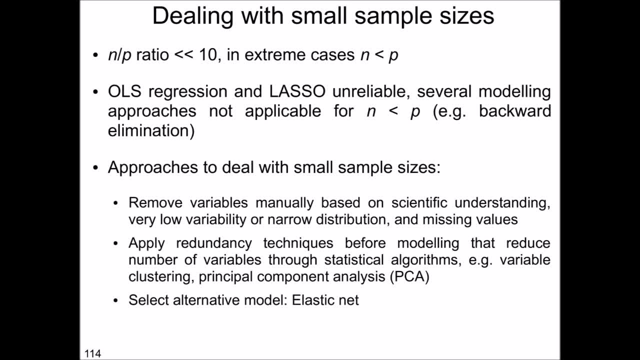 That's why you partly remove some. We will later learn about this in multivariate analysis. If you have species data where species has just been found at 1% or 2% of all sites, then it's very unlikely that you will find for the species a good correlation. 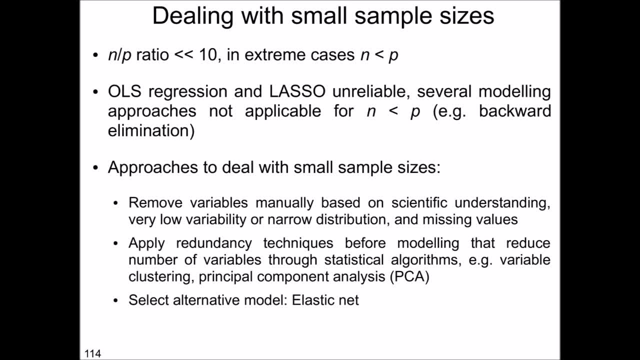 with some environmental variables. Another option is to remove variables that have many missing values, because this would actually compromise the whole analysis, Because you need to have a complete case in the analysis and you had to remove several other cases where you have values for other variables. 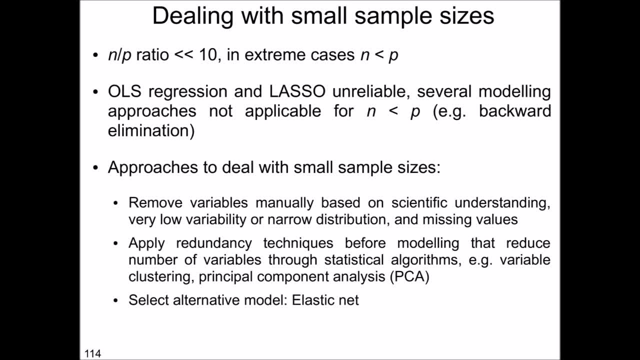 So getting rid of variables with many missing values is often a good idea. Then you can use techniques that specifically reduce the number of variables through statistical algorithms, And these are called so-called statistical algorithms. These are called redundancy techniques. For example, variable clustering can be used. 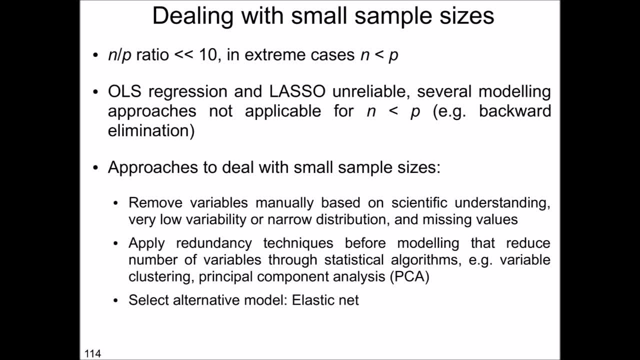 It's a cluster analysis that tries to find groups of variables, and you can afterwards use proxies for these groups and then have just a couple of group variables instead of all individual variables, And the same holds- we have discussed this before- for principal component analysis that constructs. 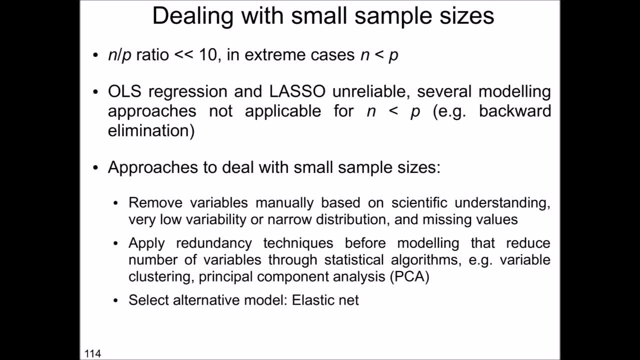 the new non-correlated variables from a data set And in the case of collinearity, this can help to reduce the number of variables, Because if you have collinearity in the original data set, then you can express some variables by the newly constructed variables. 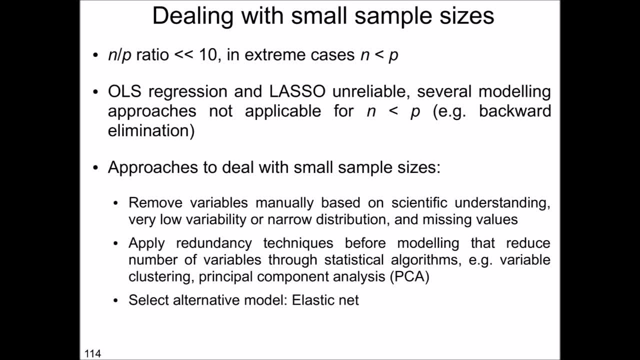 This is, for example, specifically a technique that specifically applies if you know that you have a lot of correlation between variables, and this is the case, for example, for bioclimatic variables. Many climatic phenomena are related to each other. There's a set of so-called 36 bioclimatic variable. 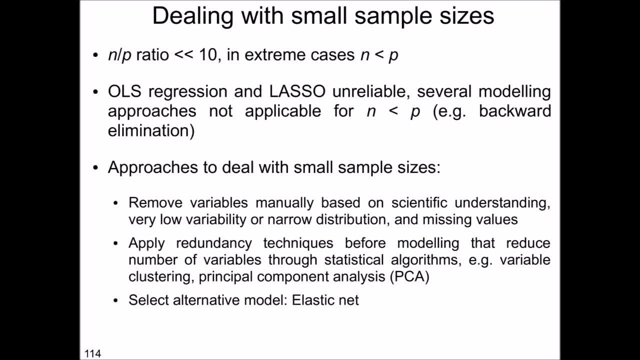 For example, these variables express spatially for different regions or how much precipitation you have: What is the lowest temperature in winter? What is the lowest temperature in summer? Highest precipitation and so on. You have 36 different variables And, of course, regions where you have very high temperatures. 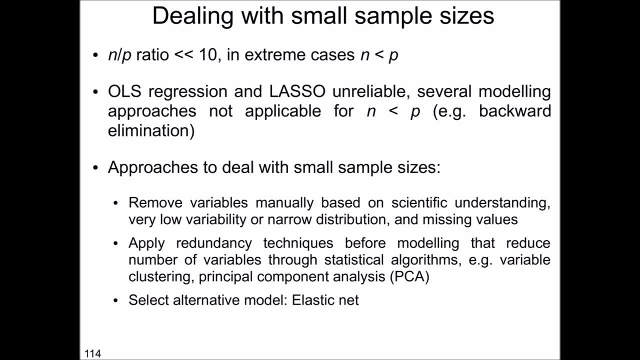 in summer tend also to have less precipitation. There are many and also relationships to other temperature variables, And these variables are often reduced by so-called redundancy techniques. In other words, you reduce the set of variables to a few principal components, So you reduce the set of individual variables. 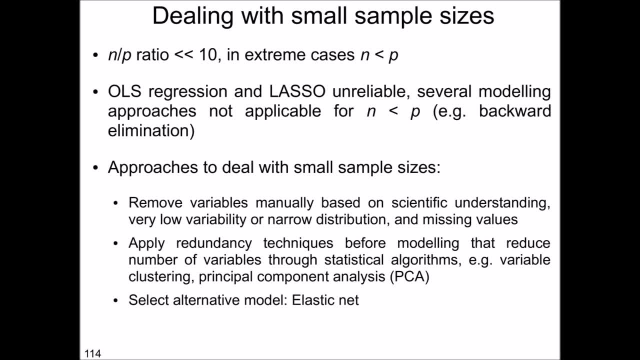 to just a few ones that are then used in the analysis. And finally, you could also select an alternative model and keep all individual variables- You do not remove some- and let this model do the job, which to some extent works, But of course this has also 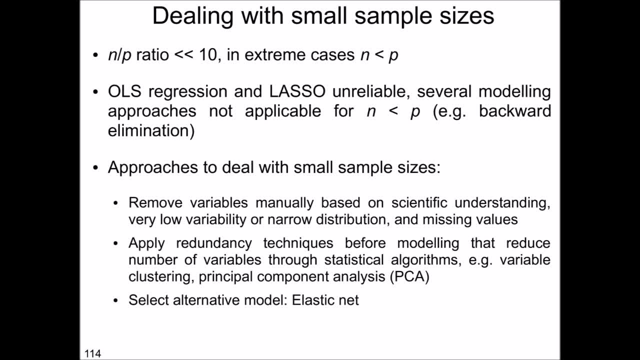 you know its limitations And that can be done with the so-called elastic net. We won't deal or go into more details on the elastic net here, but I invite you to read the paper by Sue and Hasty from 2005 on the elastic net. 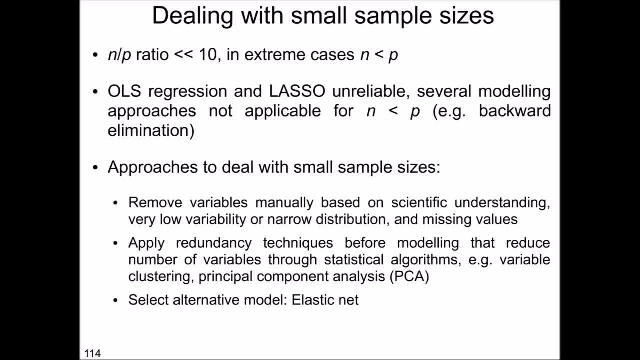 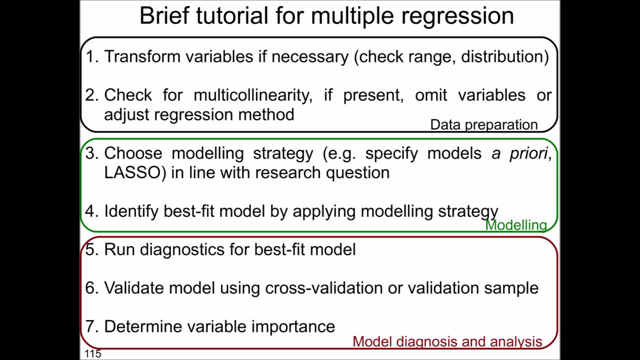 And there's a package in our with can be used to run the elastic net. Finally, we end the session with an overview of the steps that you need to do. a brief tutorial for multiple regression analysis. So first you need to transform variables if necessary. 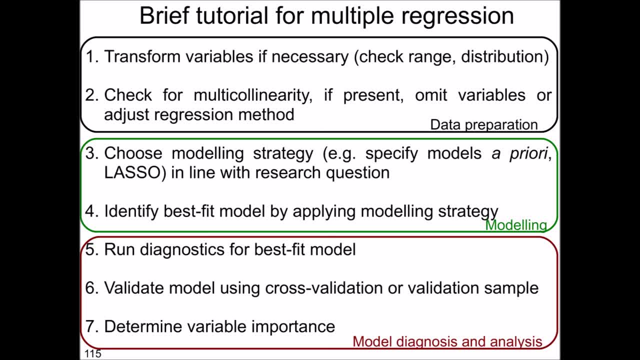 We just discussed this- Check the range and the distribution, then check for multicollinearity And if this is present on the variables- or you know it's just a regression method- choose a different model or account for this during modeling.